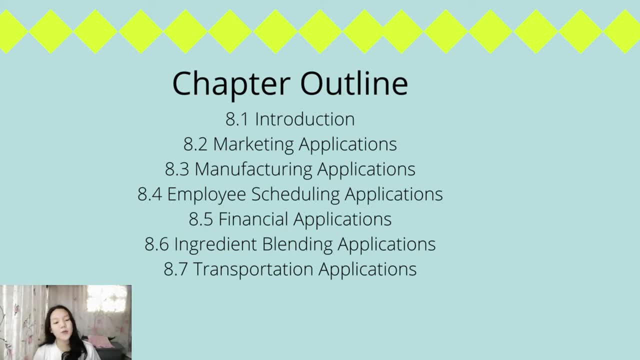 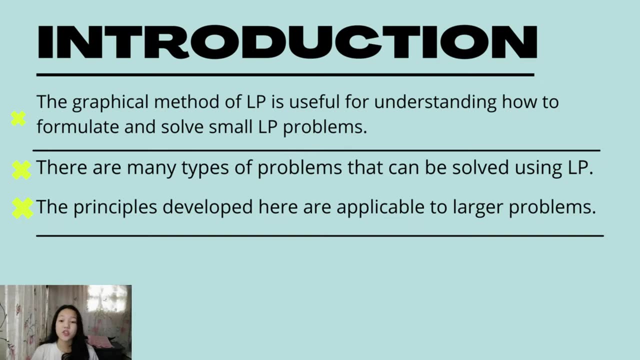 And for our last objective: today we're going to discuss about QM for Windows or the Excel Solver Software, And for our last outline we will have the Transportation Applications. Okay, so here in the introduction, we know that it is beneficial to understand or how to create and solve small linear programming issues using graphical method of linear programming. 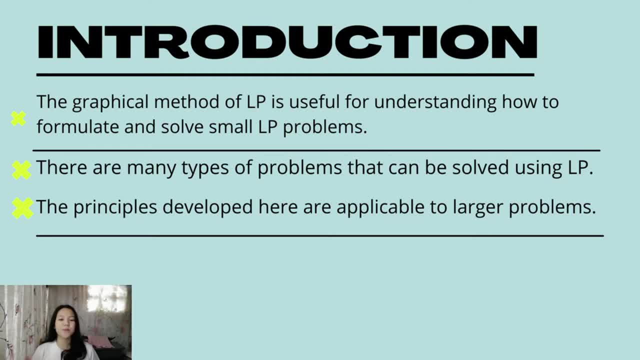 Of course, thought on the previous chapter by the previous reporter And now in this chapter. its objective is to take things further And to demonstrate how the linear programming may be used to simulate a huge variety of real world issues in general, And this can be accomplished through the presentation of examples of models in the fields of marketing research. 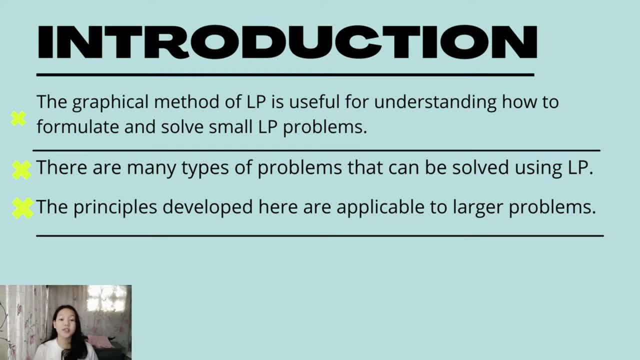 in the fields of media selection, production mix, labor scheduling, production scheduling, shipping and transportation for the ingredient mix and the financial portfolio selection, among other topics. So we should know that this linear programming tool is used in business and industry for a variety of tasks. 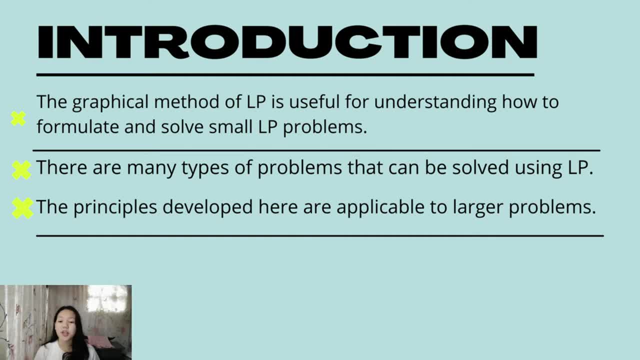 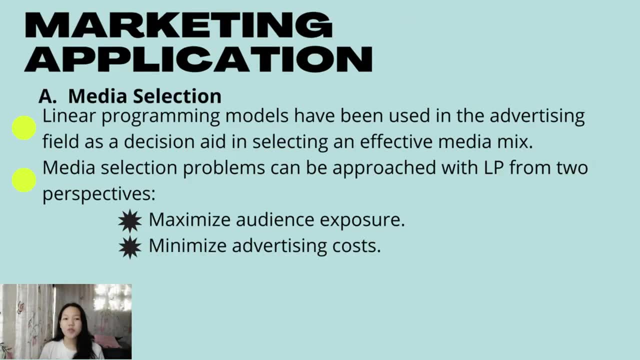 such as production planning, transportation and routing and many sorts of scheduling. And among all its applications we have here, the first one is in marketing application. Under the marketing application we have two. The first one will be media selection and the second one is the marketing research. 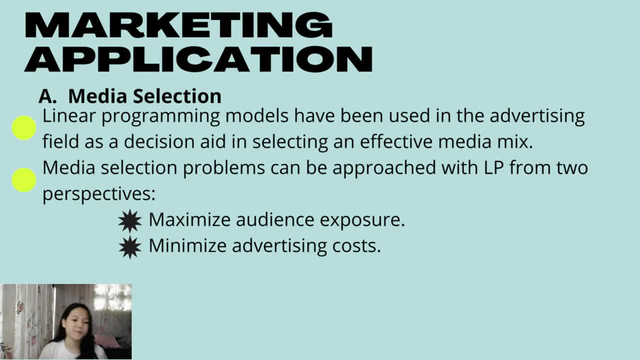 but we'll now only focus to media selection Here. in media selection, the linear programming can be used to solve challenges involving media choices from two different angles. So we have to look forward to either objectives which are to maximize the audience exposure and to minimize the advertising cost. 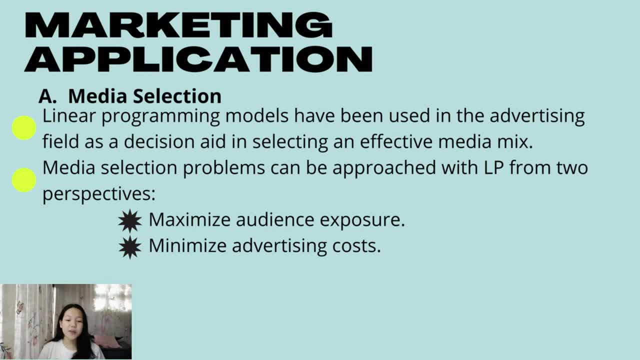 So, as a decision aid in advertising business, the linear programming models have been employed to select a successful mix for a number of years, So it has been used long, long time ago. I mean, yeah, it's been used now already, And some companies use this strategy when allocating a fixed or limited budget across numerous media. 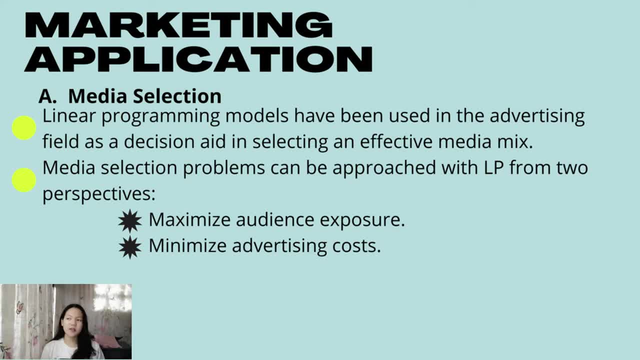 which may include the very common types of media Which actually we're still using for today is television, And then radio spots, newspaper ads, magazine advertisements and other forms of marketing communication, And in other application the goal is to maximize its audience exposure. 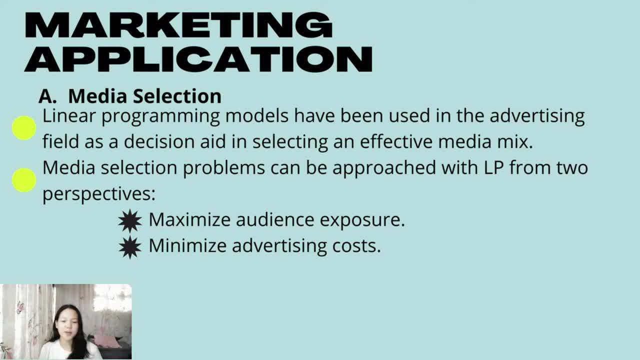 That's what I have mentioned earlier And of course it will also be used for marketing purposes. And of course it will also be used for marketing purposes also vary in different terms, so it depends on the circumstances, it depends on the contract requirements and it also depends on the limited media availability. also, it depends, of course, to 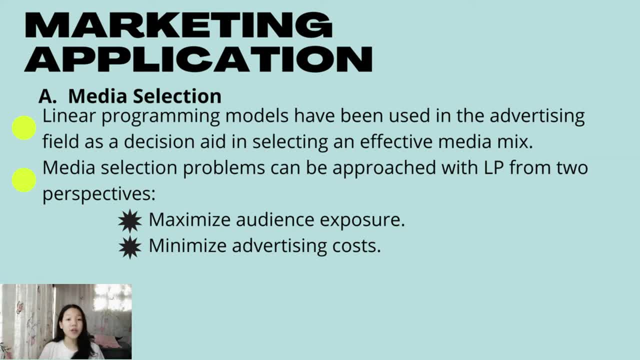 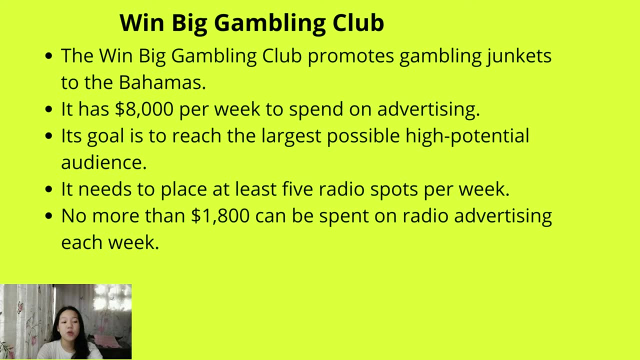 the policy of the company, if ever they want to. you want to impose restrictions on the permissible medium mix. so that's how it may vary. and now and now, let me give you another good example, whereas the linear programming is used in media selection. so we have here the situation regarding 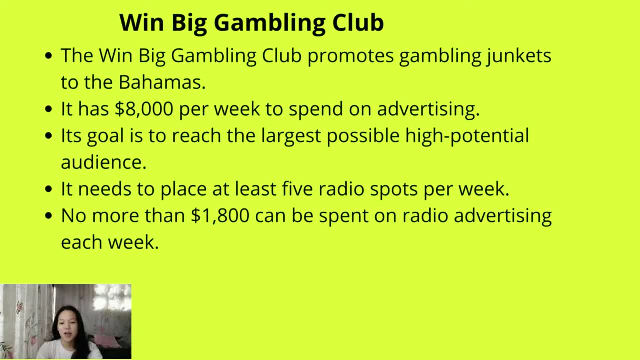 the win big gambling club. so here we have- i know we have here the things which is required when solving or maximizing its total reach of- i know, total reach of audience, you know objective and before we achieve those, here are the things needed to be done or needed to be complied. the win big gambling club promotes. 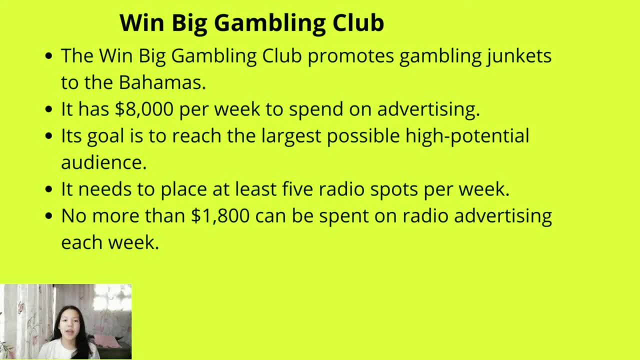 gambling junkets to the bahamas and it has eight thousand dollars per week to spend on advertising and its goal, as i have said earlier, its objective or its goal is to reach the largest possible high potential audience, and the media types and audience figures are shown in the. 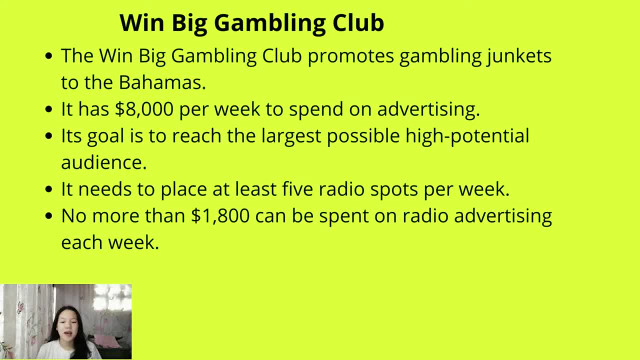 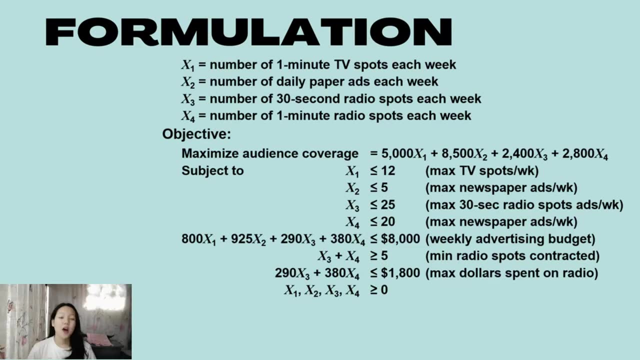 following table on the next slide: and it needs to place at least five radio spots per week. i mean, the advertisement needs to place at least five radio spots per week and no more than one thousand eight hundred dollars can be spent on radio advertising. okay, so we have. okay, so we have. 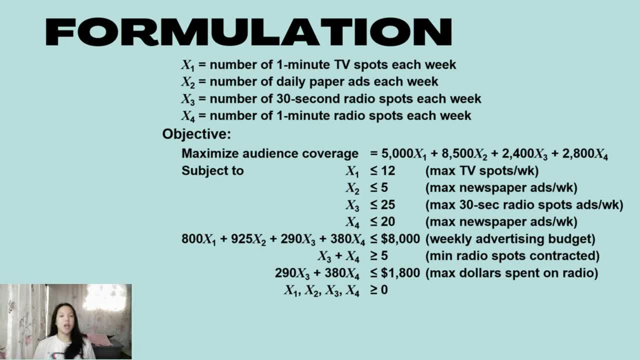 here in formulation and uh representation of different media, from x sub one to x sub four. x sub one is the number of one minute tv spots where the advertisement will appear and x2 is where the newspaper ad or the advertisement will appear in the newspaper. added the x sub 3 and x sub. 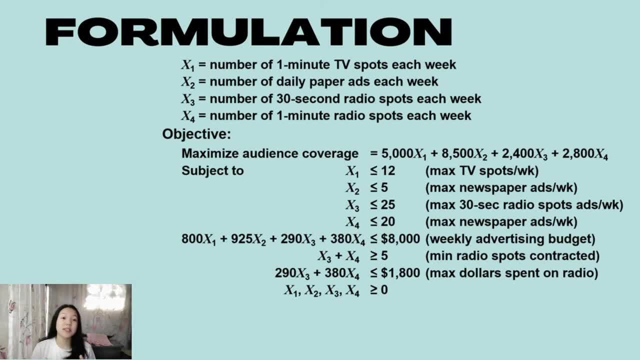 4 for the two different radio spots and of course, its objective is to maximize the audience coverage, which is equal to the sum of the audience reach per media corresponding to the to the media where it should appear. so we have here the 5000 times X sub 1 plus 8500. 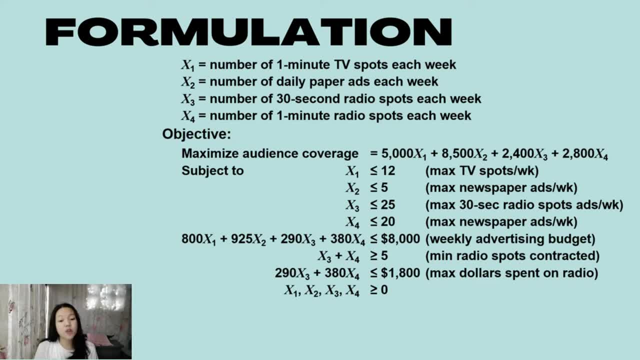 times X sub 2, plus 2400 times X sub 3, and then the 2800 X sub 4, so these will all be explained on the next video that will be shown, a tutorial video using our Excel solver, and then we have here, of course, our constraint. 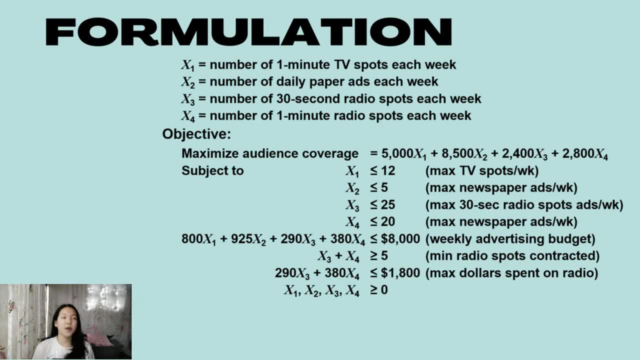 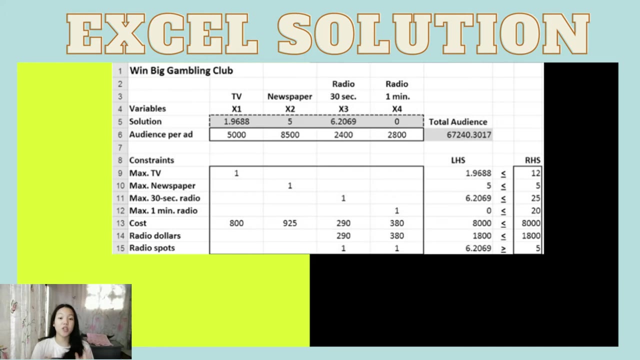 these are subject to or constraint, by which is I mean the constraint is where our restrictions, or it is things are limited to. so subject to ganon, ganon, ganon. and in the next and for the next slide, here is our Excel solution: dito ipakita niya na, solve niya na. pero I'm going to show a video to you. 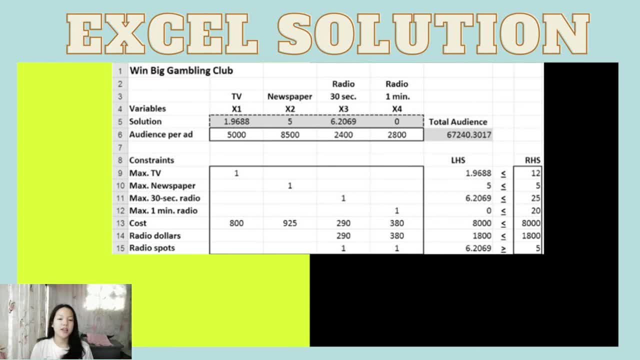 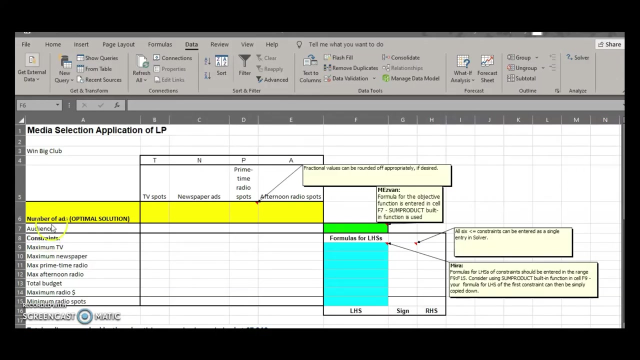 which is a tutorial video showing how did it arrive to this answer. so I hope you'll focus on your screen and listen so you could appreciate and- a good, you could actually know how to use the Excel solver software, because it helps a lot. okay, let's play the video. so we're using a software in Excel to solve the win big. 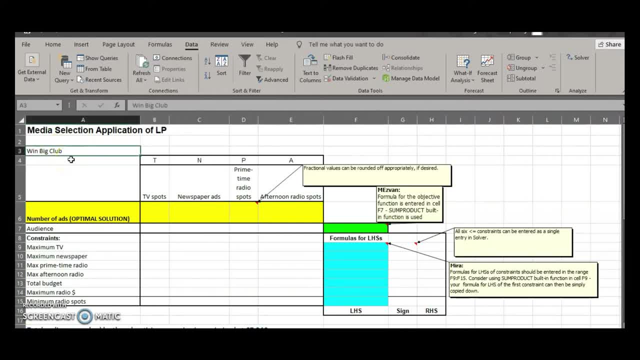 gambling club problem. basically, we have four different choices of medium for which to advertise, which are the TV spots, newspaper odds, primetime Radio spots and the afternoon radio spots. we also have constraints, so, given these both restraints, cost and the budget, what we want to know is how many of each type. 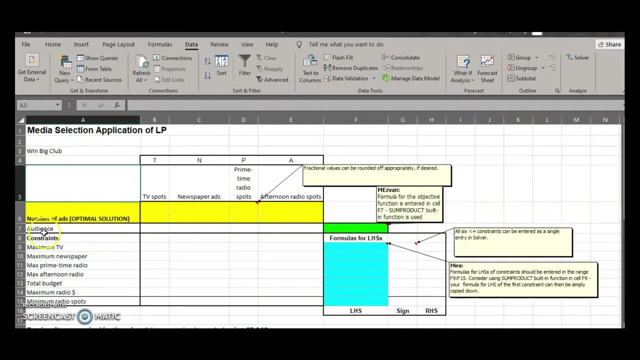 of spot we should run to maximize the audience that we're going to reach. the first thing we're going to start by filling in is how many people we'll reach with every TV spots, newspaper ads and within the two Radio spots好, Now let's talk about what we're doing. let's run both sites. 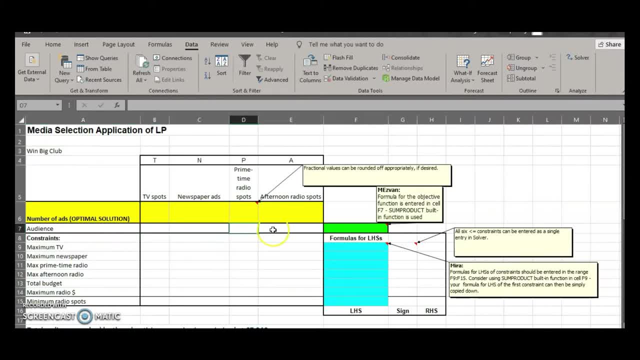 we're using this data and we went over the top of the list, which is your. with this chart, we have two ones, or two in total: 1 sticky notes〉 & 2 boxes on the line 2 helpful things for us〉 & also these are things like those sheets. 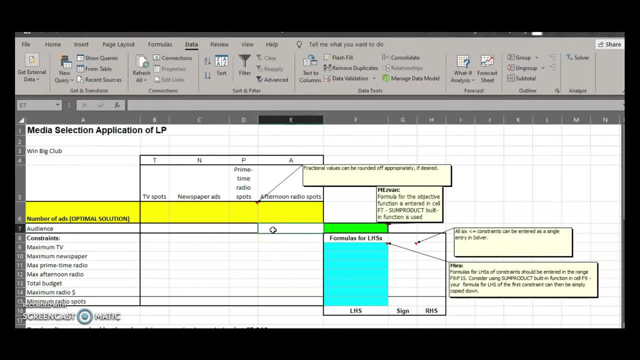 like this, big вспfires, is going to be a must to set up as side notes Favorite. Now what we're going to do is write the formula of the objective function. What we want to know is, given that we run a certain number of TV spots, 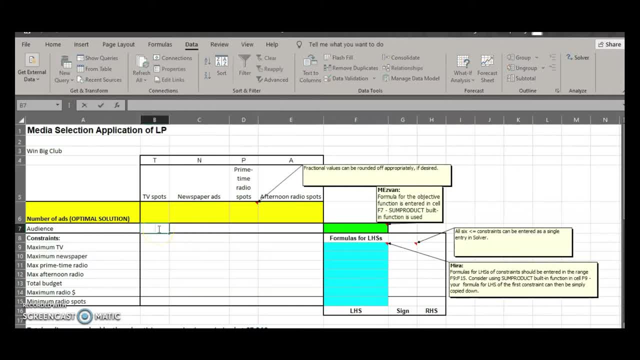 and each TV spot is going to give us an audience of 5,000 people, plus however many newspapers we run, multiplied by 8,500 people, plus the number of primetime spots we run- times 2,400 people, and then the number of afternoon spots- times 2,800 people. 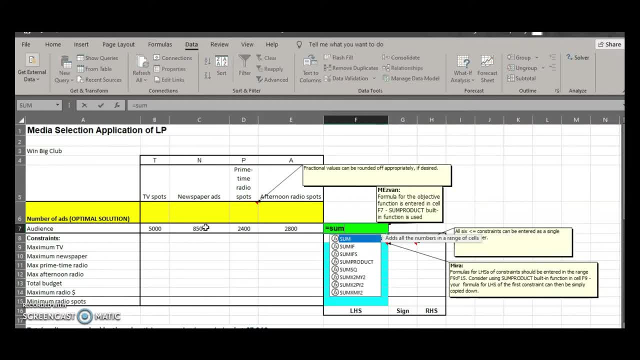 Okay. so the way we're going to write this formula is with some product and take this range and say we want to multiply these items by these items. so it's going to be from cell B6 through E6.. And from cell B7 through E7,. 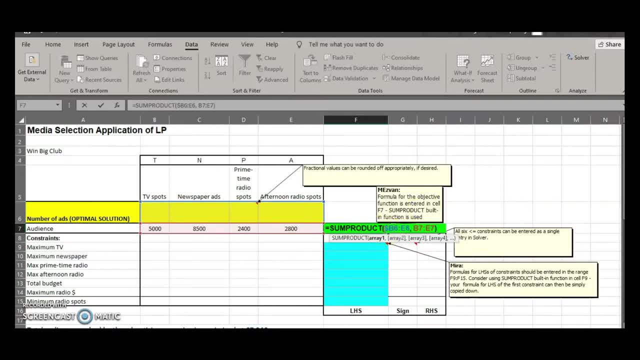 but by making the B6 through E6 as an absolute value, by adding dollar sign into it. And now we're going to copy this formula for all of the other constraints. I'm going to copy this and paste it here, And then the next thing we're going to do is to write down our constraints. 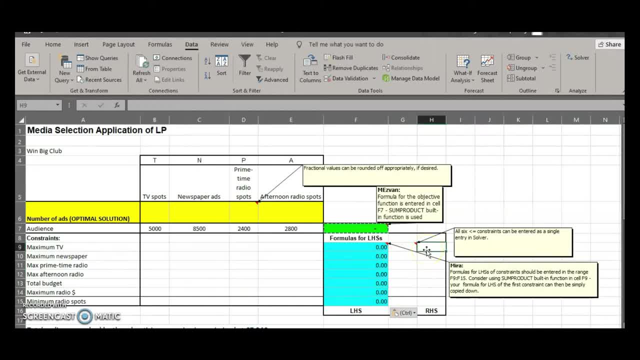 We have been told that the number of maximum TV odd that we should run in a week is 3,000.. So that's 12.. So why didn't we fill that in first And for this to be less than or equal to 12,? 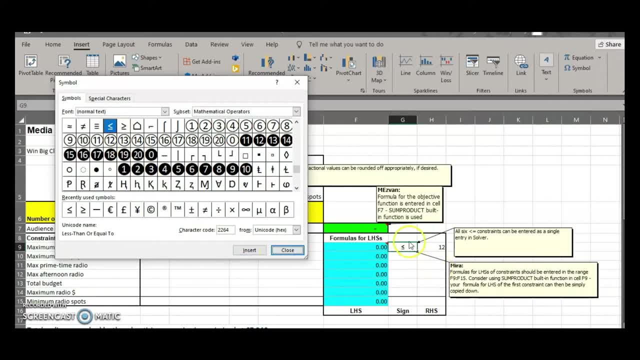 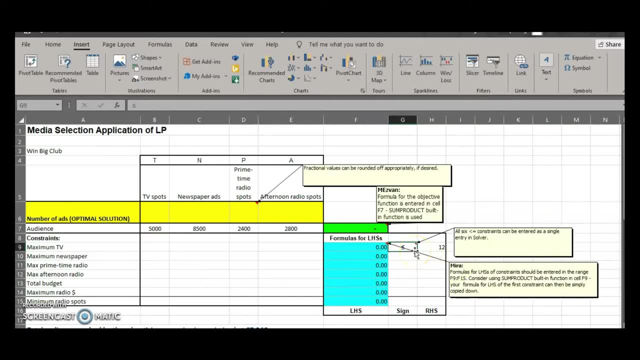 so, taking the value of whatever is in B6, wanting that to be less than 12, we'll write that as putting a surrogate here. Well, a surrogate is a function that approximates another function, For example, to search for a point that minimizes an object function. 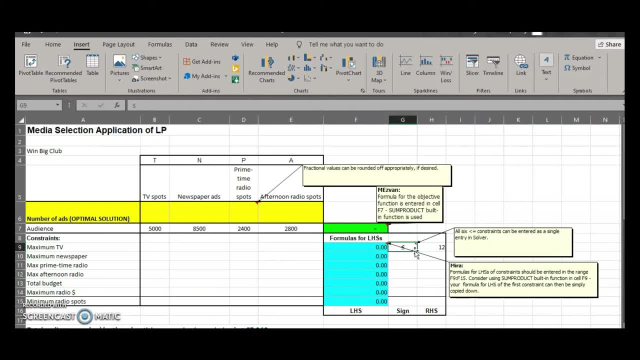 simply evaluate its surrogate on thousands of points and then take the best value as an approximation of the objective function. and we're going to put number one here. so you'll notice in its formula that the number of tv spots multiplied by one, added to the number of newspaper ad that we run. 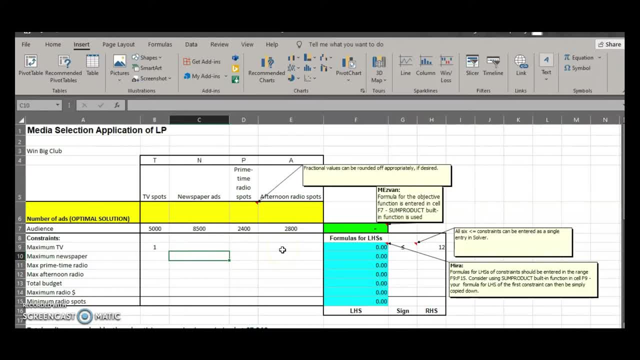 multiplied by none. same goes with the next two medium and this, this will give, you will give us. the number of tv spots has to be less than or equal to 12, and for the maximum newspaper ads- we've been told that it is five- the maximum number of. 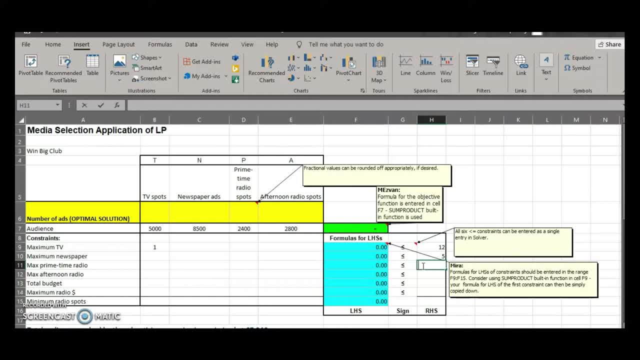 prime time radio spot is 25 and the maximum number of afternoon radio spots is 20. and now we're going to deal with the budget constraint and it has to do with how much money we have to spend. so we have to spend less than or equal to eight thousand dollars. it's eight thousand dollars. 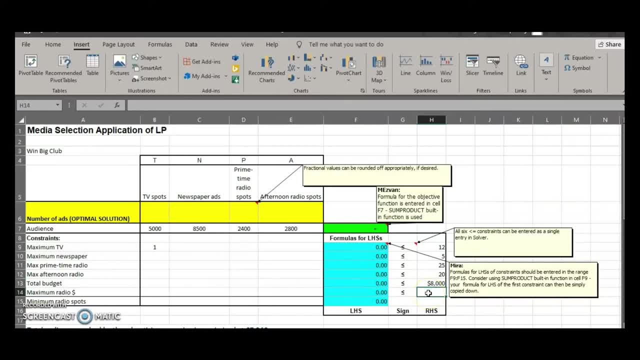 and we're not going to use one anymore in using this constraint, because now we're talking about how much are we spending? and it costs eight hundred dollars to run a tv spot. so we take the number of tv spots we're going to run, multiplied by eight hundred thousand. 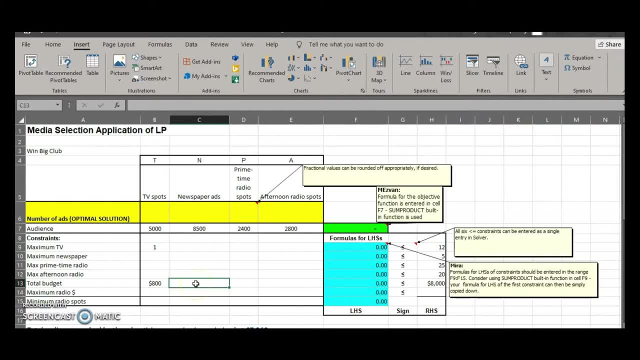 eight hundred dollars per ad, plus how many newspaper ads we're going to run- times, the price of the newspaper ad- and we're going to use the number of tv spots that we're going to run, and so on. so the price of the newspaper ads is nine hundred and twenty five dollars. 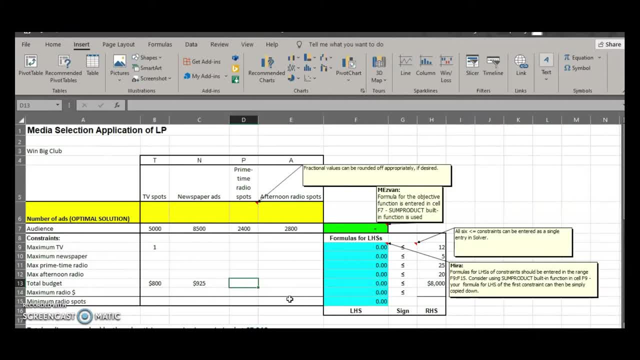 while in prime time radio spot is 290 dollars, also given in the afternoon, radio spot is 380 dollars. we've also given a constraint and the amount of money that we can spend on radio ads and it has to be less than or equal to one thousand and eight, one thousand and eight hundred dollars. so again, 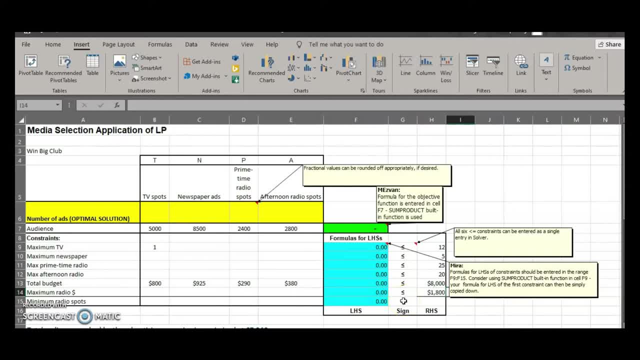 as we are talking about the cost, the money, the amount of money for spending on radio ads will also be 290 dollars and 380 dollars respectively. okay, so notice that we put all of our less than constraint all together and our last constraint is a greater than constraint. 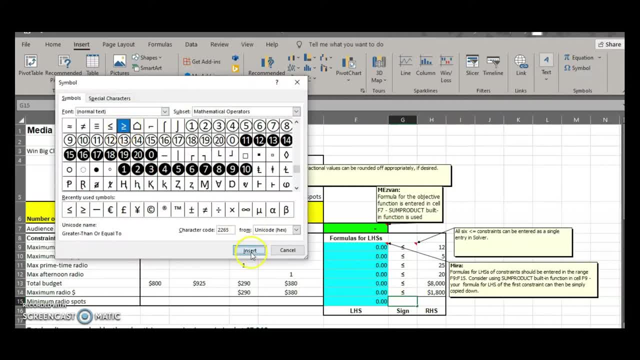 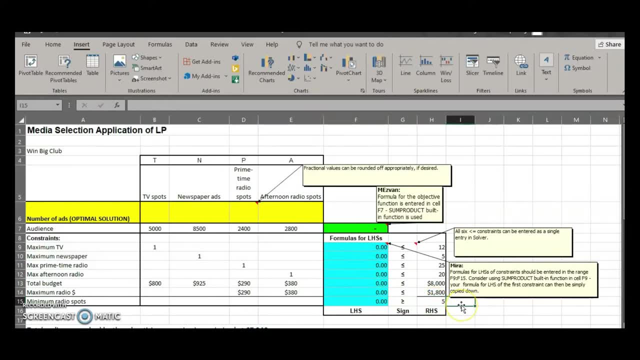 here we've given a minimum of radio spots we should have in a week, and that is at least five radio spots. it's five or more for what it means. so, talking back about the number of radio spots, we then again want to use the value of one multiplied by the number of prime time spots plus. 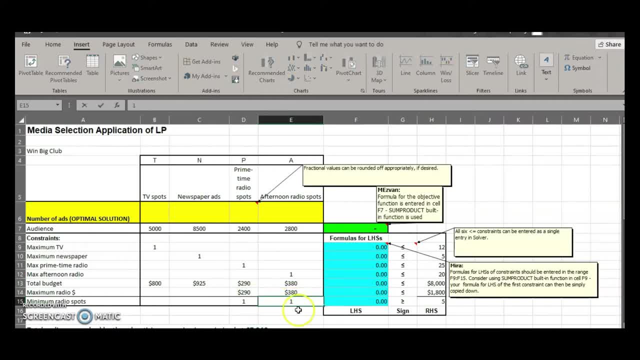 one times the number of afternoon spots to be greater than or equal to five. so now, as we complete our data, we are ready. we are ready to use the solver. you have to go to the data tab, go to the data tab and then click the solver. you have to click the solver and then you have to add all of this needed information. 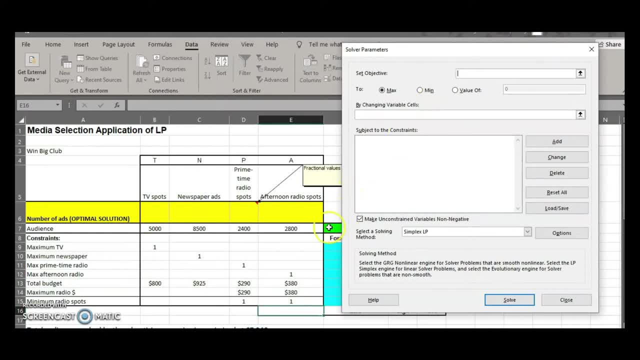 the objective function is in cell F7, so it has to be the cell F5, because that's the number of people that will be reaching, wanting it to be maximized. so the changing variables are from from the cell b6 through a6. okay, so now, after that, we're going. 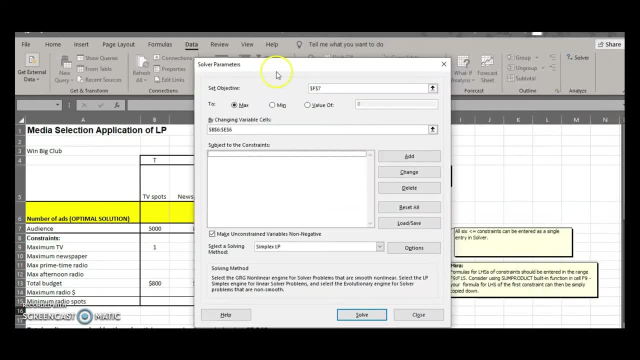 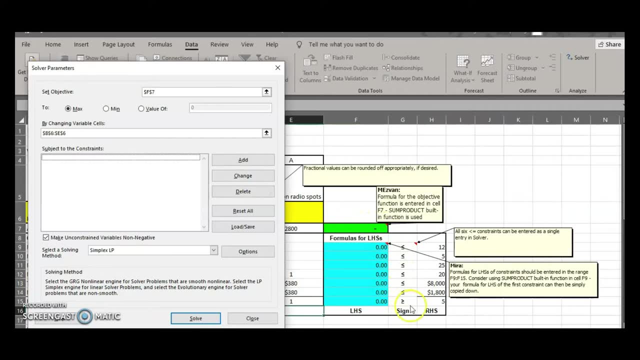 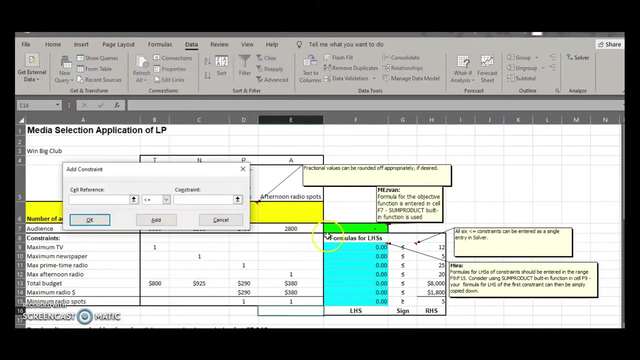 to input our set of constraints, keeping all together the less than constraints and then the greater than constraint, because this way, in separating those, it allows us to enter this constraint as a block and not adding it individually. okay, it's time to click the odd. click the odd and then you highlight the cell that has less than constraint. okay, we have to highlight. 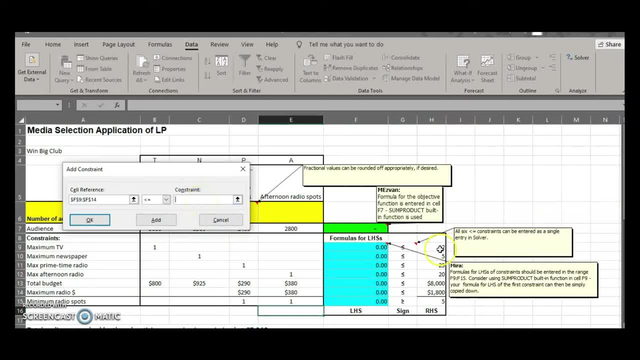 the cell that has less than constraint. and then you highlight the cell that has less than constraint. that has less than constraint and you want to set it constraint to the value of h9 through h14. okay, click add again. and then now let's add another greater than constraint. 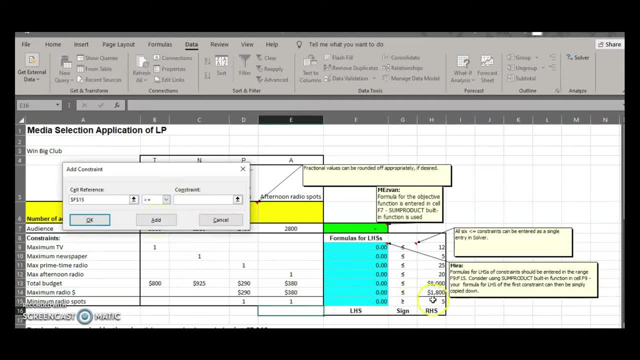 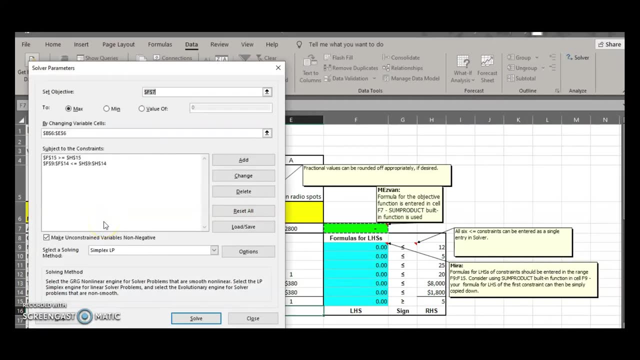 let's add a greater than constraint following, following the same input process. but of course, but of course you could add more constraint if given any, but here, because this is our last constraint, we will press okay. let's have to press okay and then click here: the make the. 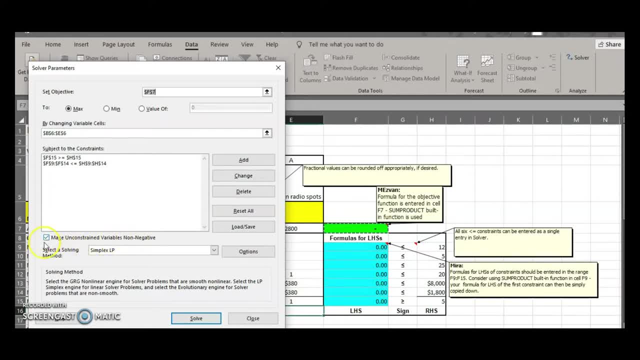 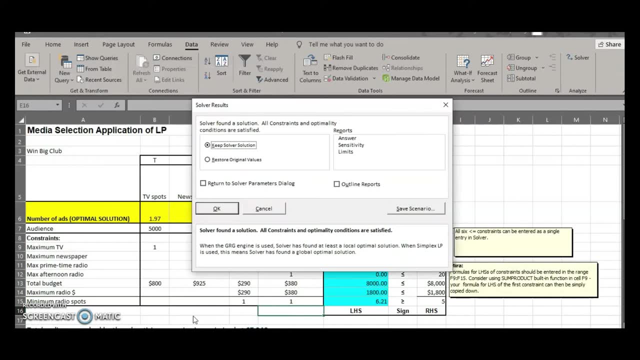 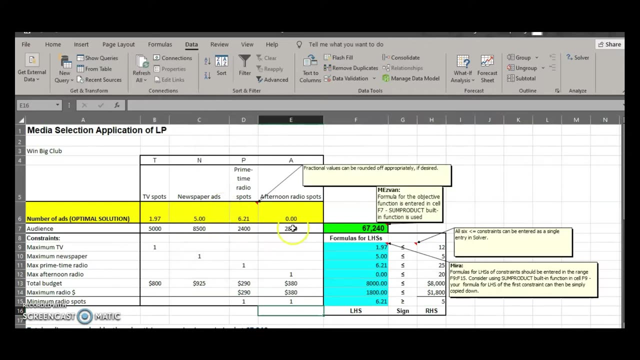 unconstrained variable, non-negative, and right after that we have to solve this. click the solve and then this will show you the results. okay, these are the results that been solved by the excel solver software itself, but these values could be rounded off if the side of making it a whole number by that you 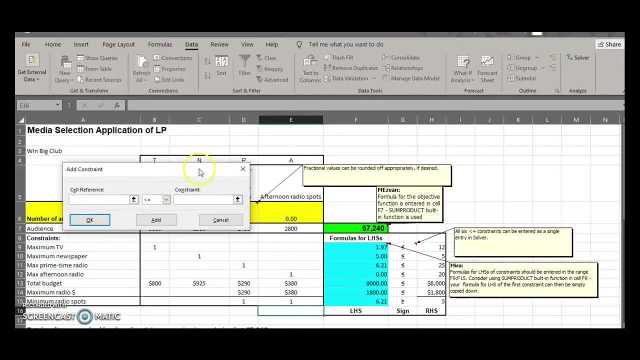 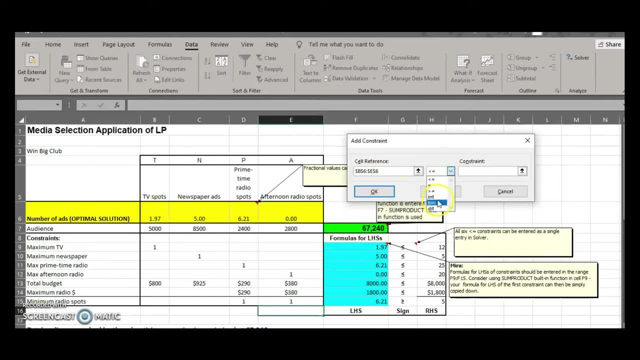 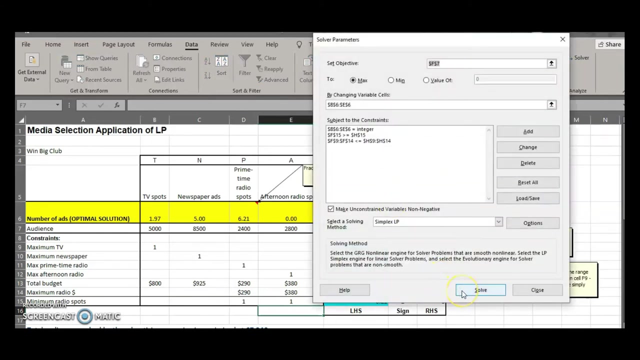 have to add another constraint and put it on integer. if I just have to add another constraint here and you have to put it into integer, because it means that a fractional value is not an option here and will result only on to whole numbers and this whole numbers will be resulting to a more accurate 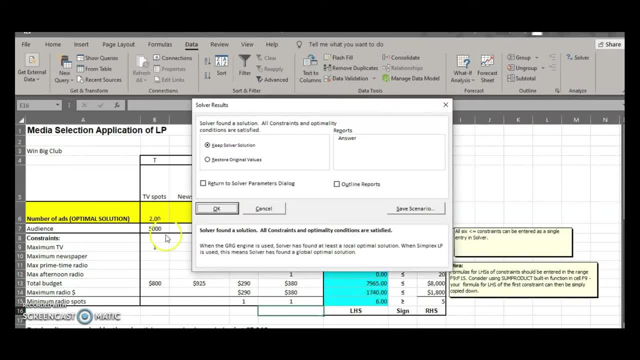 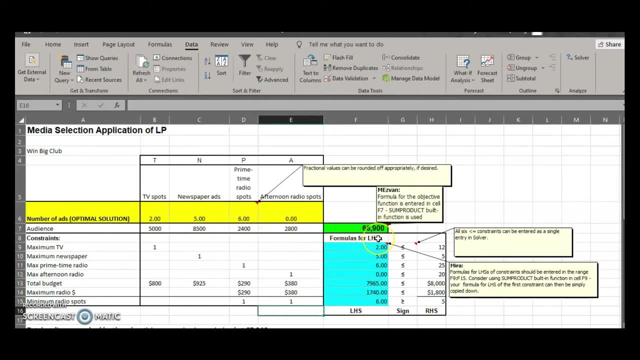 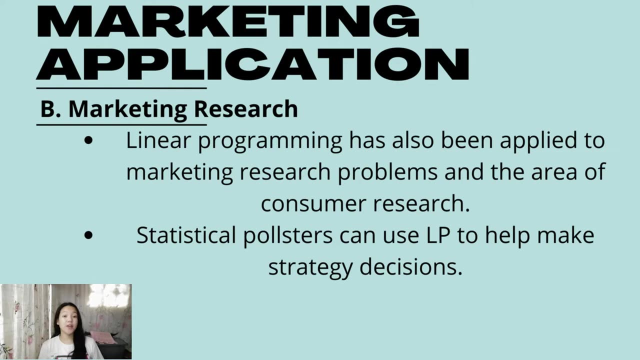 results. okay, now, after you put the integer, it shows whole numbers at as its value. okay for the second application for the marketing is. we have here the marketing research. so it's the linear programming has also been applied for the marketing research and for the area of consumers research and make marketing research is. 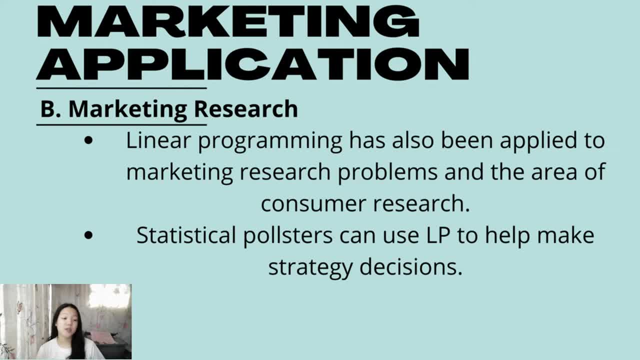 a scientific process that commercial organization organizations use to acquire information and that there mean that requirements and wants of the customers, as well as the most effective, effective methods of meeting those needs and wants while maintaining the long-term profitability. the objectives are to provide a business organizations with the ability to fine-tune the marketing mix and in order 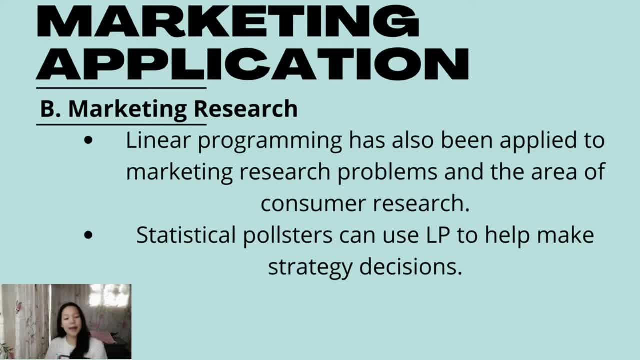 to in order to better address consumer requirements and expectations, while maintaining a balance of life for products. in response to the customers demands, and the appropriate decisions may be made at may be made at the satisfaction level from the top and the bottom spider bank. examples of marketing certifications and constraints based on the수. 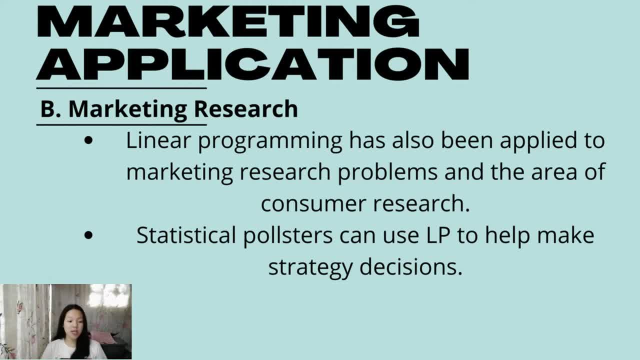 research מח Split校 and operational levels using the right market research should be콜 Dancing, with the help, of course, of the descriptive, diagnostic and predictive research at the steady check and operation of levels using the right market research information and it is possible of an organization to benefit. 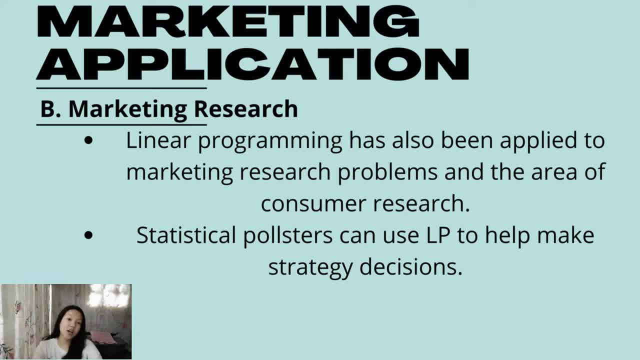 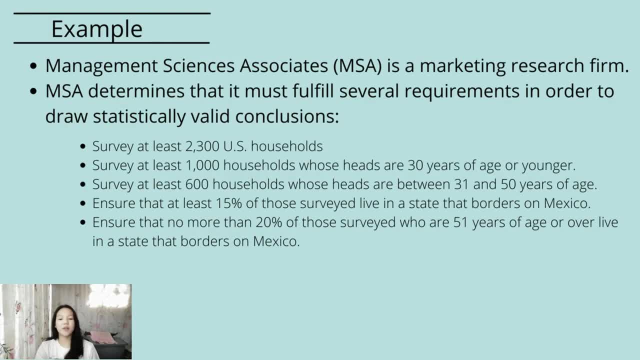 uses or optimizes the linear programming model. so let me give you a real-life example of it. so here is a management sciences associates, which is a marketing research firm, and here are the things or the requirements needed to be done or to achieve in order to solve for its. 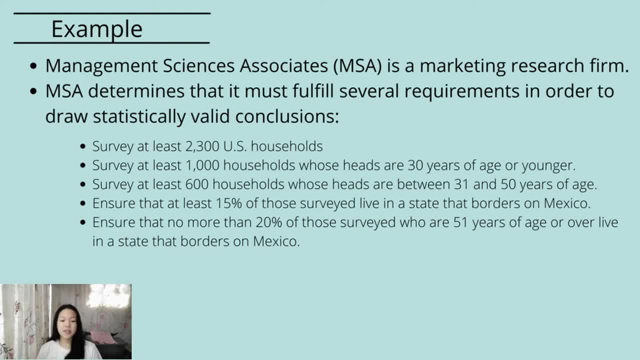 missing piece. the msa determines that it is must fulfill. it must fulfill several requirements in order to draw statistically valid conclusions. so, in order for it to be valid, this should be followed, the survey at least, should at least be 2,300 us households and that the survey should 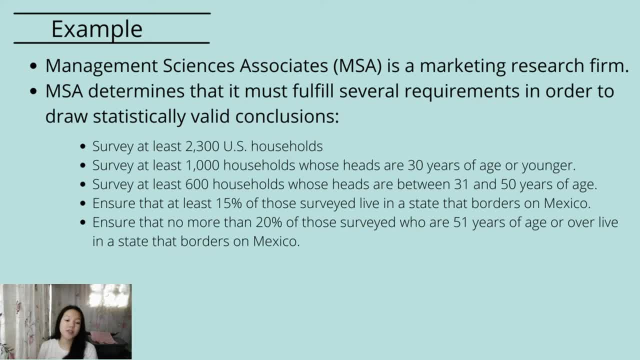 be at least 1,000 households whose heads are 30 years of age or younger, and the survey should at least be 600 households- households whose heads are between 31 to 50 years of age- and to ensure that at least 15% of those surveyed live in a state that borders on Mexico and another. 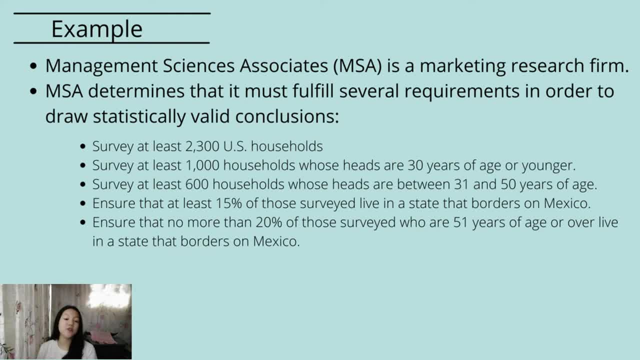 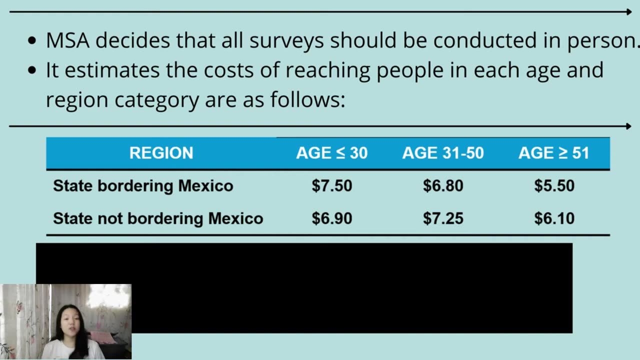 one is that they ensure the no more than 20% of those surveyed are 51 years of age or over lived in a state to border on Mexico. so here shows the table. yeah, people show. Backchaяти would show three differences for presidentKyoto Mfun: to and and from, Or can you say what is different? 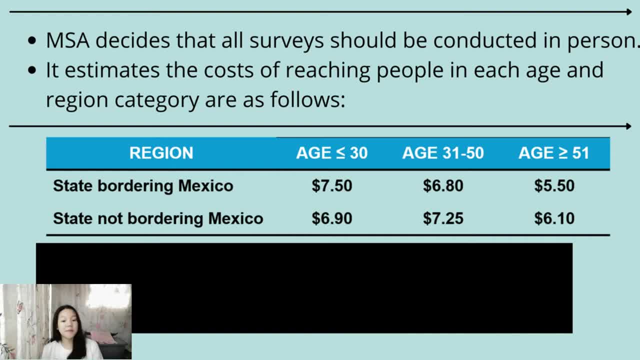 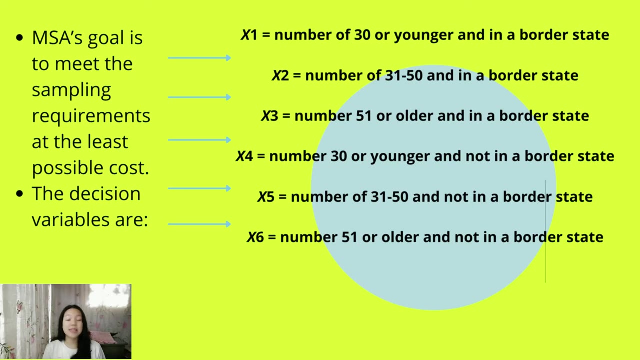 different region, which is bordering and not bordering in mexico, and of course the bracketing of age to the specific surveys in the specific range of age. it has of course different costs here. the msa's goal is to meet the sampling requirements at the least possible cost, so here we have to minimize our cost, of course. 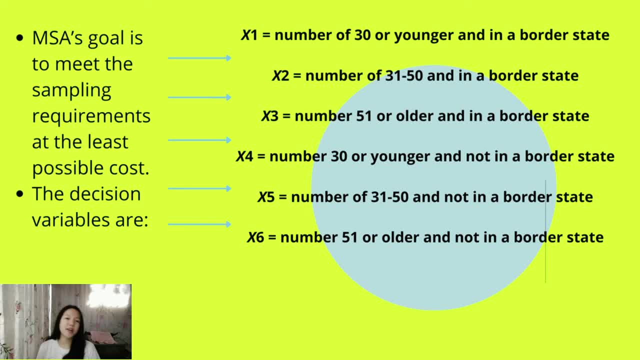 and the decision variables are present. decision variables represent from x sub 1 up to x sub 6, representing the number of ages in a different regions. in different regions, different ages range, where they belong and, of course, if where they belong to any of those two regions. so 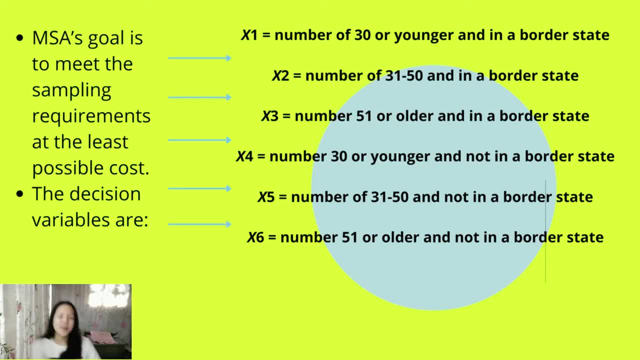 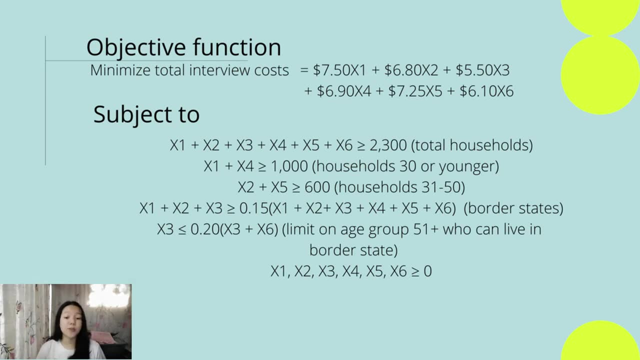 just reading this so written on the screen. i mean, is the representations of variables, of course, needed to be input? i needed for the data on how to solve it on the excel. and here our objective is to minimize total interview cost. is what i have said and it is. 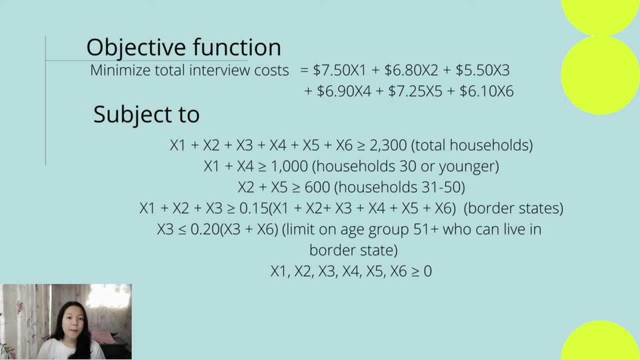 the total cost per total cost per survey in a specific, in a specific number of ages or number of ages and regions where they belong, representing, represented by 7.50 x sub 1 plus 6.80 x except 2 up to the 6.10 x sub 6, and it has this specific constraints also. 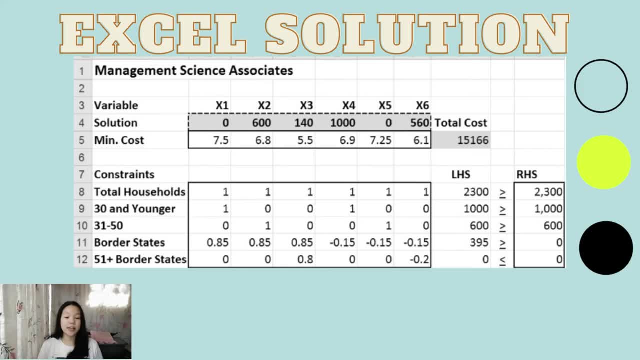 so, given the constraints, and then for its excel solution is: it is here, it's here and the same process of solving, just as how we solve for the media selection. So if you've watched a tutorial and then you've learned something from it, it is also that. 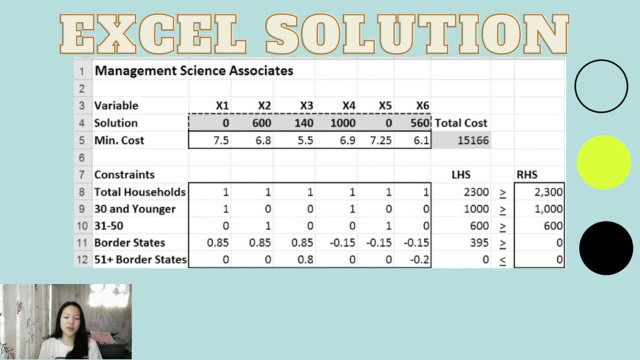 easy to solve this marketing research. So that's how easy it is, because the data you need, the data, the constraint, the constrictions, variables, solutions and, of course, it's objectives, and all you have to do is to input those. 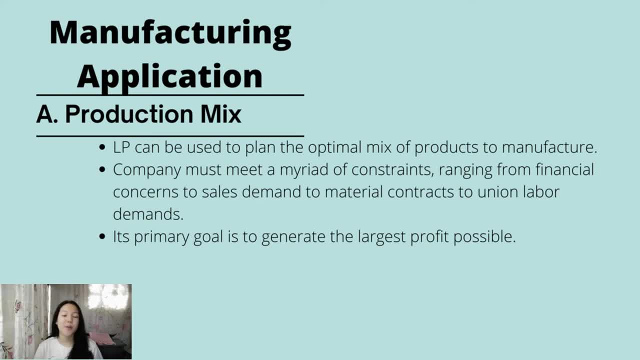 And now we are down to our second application, which is in manufacturing applications. We also have two items under the manufacturing application, which are: the first is the production mix and the production scheduling. First we are going to discuss the production mix. So the total set of products or services offered by a company is referred to as production. 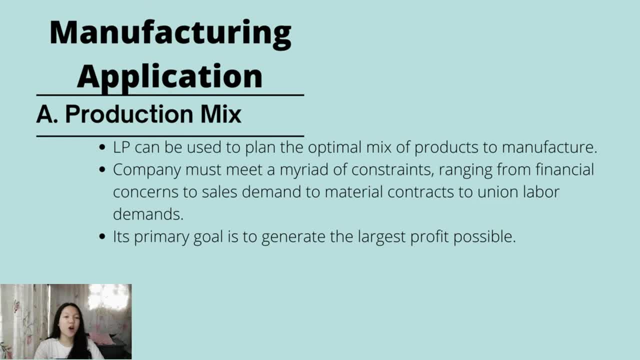 mix. The product mix, also known as the product assortment or the product portfolio, is made up of product lines which are related, things that consumers tend to use together or think are similar to one another And, in terms of products or services, a fertile field for the application of linear programming. 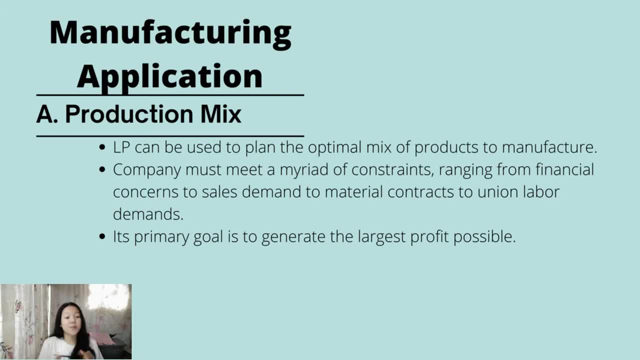 is the process of determining the appropriate mix of products to be manufactured. So managing a company's operation means dealing with a wide range of constraints- from financial considerations to sales, to demands and to the material contracts, to union labor and demands- And its major objective is to earn the greatest amount of profit possible. 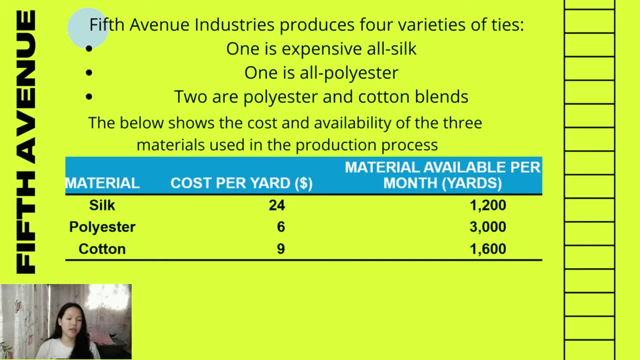 So given here an example of the Fifth Avenue industries. So we have a linear situation, which is it has the four varieties of ties. So let's talk about ties in this time: One expensive, old silk, one is all polyester and two are combinations of a polyester and 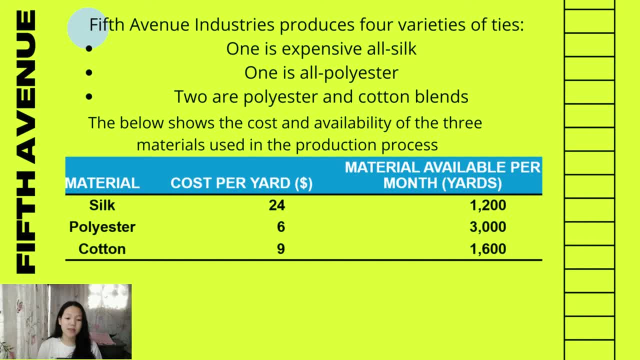 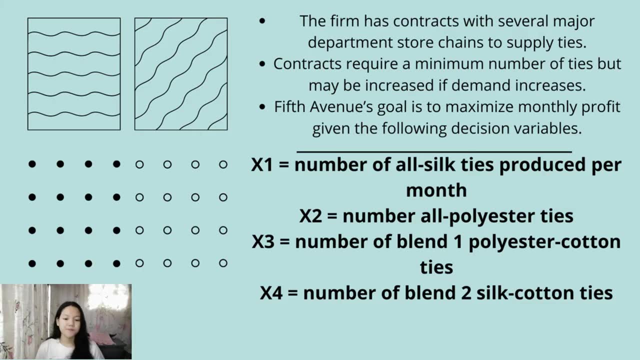 cotton blends Here on the table. it shows the availability of the three materials used in the product process. We have silk, polyester and cotton, and we have here the cost per yard and of course the material available per month. Here we have also the different variables. 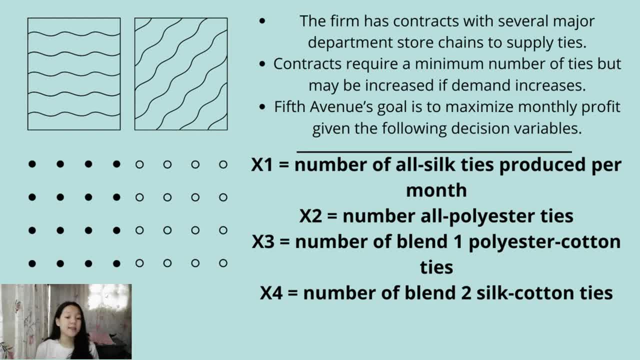 The firm has contracts with several major department stores chained to supply ties And the contract requires a minimum number of ties but of course maybe it could increase. It depends on the demand And the Fifth Avenue's goal is to maximize monthly profit. 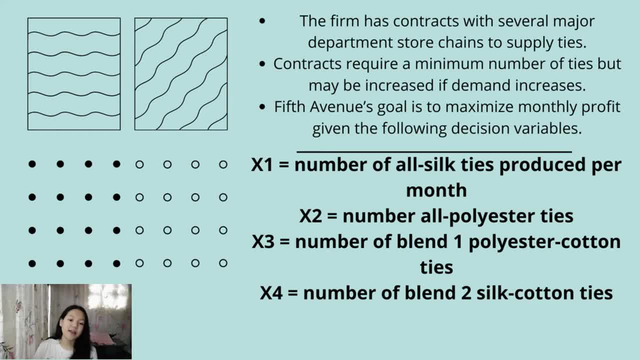 Given the following decisions. So here are the variables: X sub 1 to X sub 4.. For X sub 1, you have the number of silk ties produced per month. X sub 2 is the number of all polyester ties. X sub 3 is the number of blend 1 polyester cotton ties. 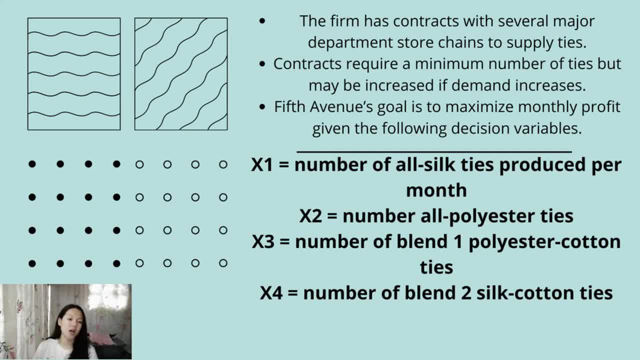 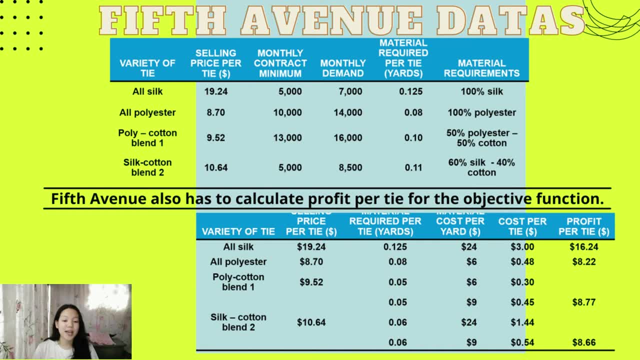 And X sub 4 for the number of blend 2 silk cotton ties. Here are the data of the Fifth Avenue Of course, composing of the selling price per tie, the monthly contract minimum- because they set a contract with their retailers- And monthly demand. 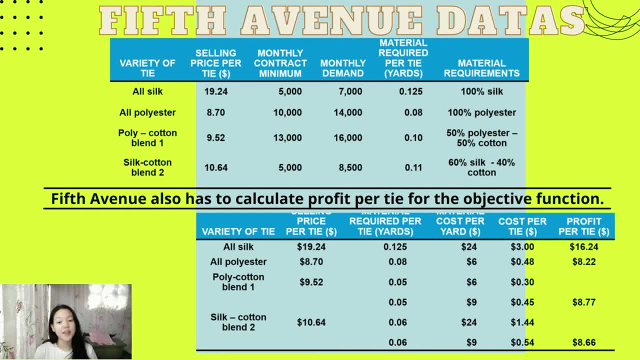 Of course, because the demand per month of the ties is different. So we have here the data And the material required per yard. So it's cost for the material required because it's different. And for the material requirements is if it is 100% silk, if it's 50% polyester or 100%. 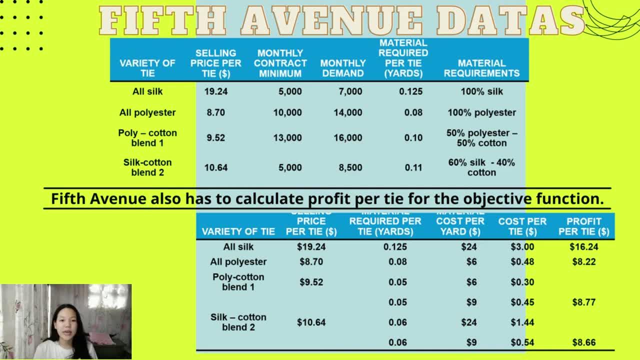 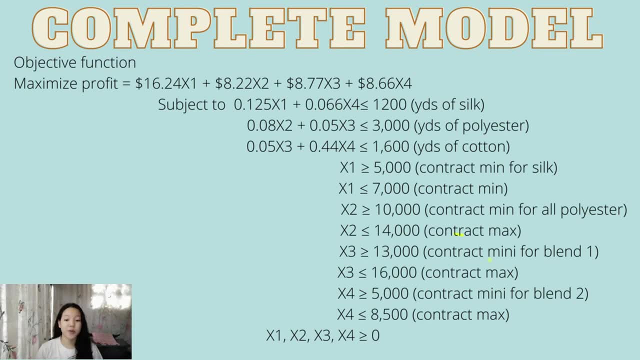 polyester or 100% cotton, 50% cotton. So here it is being pulled And of course, for us to solve for the objective of this Fifth Avenue industry, we have to also solve for the profit for each tie. So per tie given in the table, on table number 2 on the last column, will be $16,, $8,, $8, and 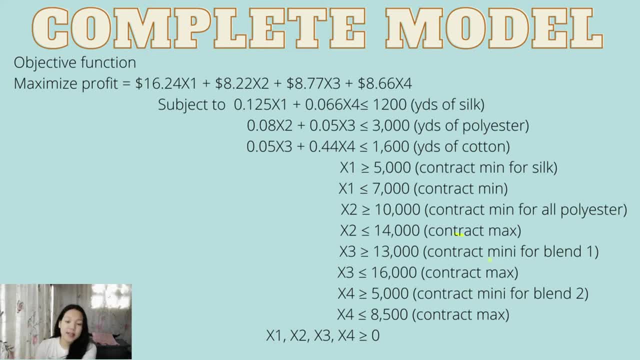 $8.. So showing here the complete model, Because this is the objective. The objective of this is to maximize the profit. So it represents, or it is equal to the sum of the profit per tie multiplied by the or corresponding to the different variables stated earlier: x sub 1, x sub 2, x sub 3, to x sub. 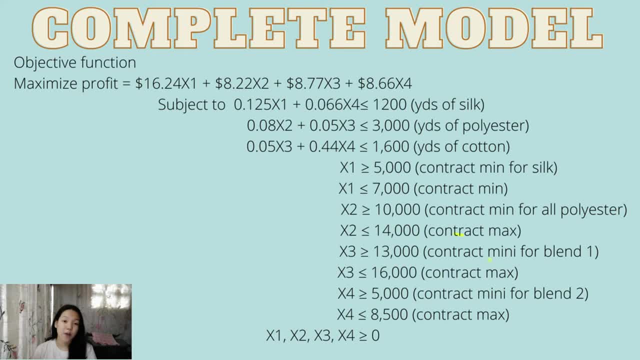 4. So they have representations which are the numbers of polyester tie, numbers of silk, numbers of cotton, And then, of course, the constraints will not be removed, which is also important. Here it is shown on this model And here is its Excel solution. 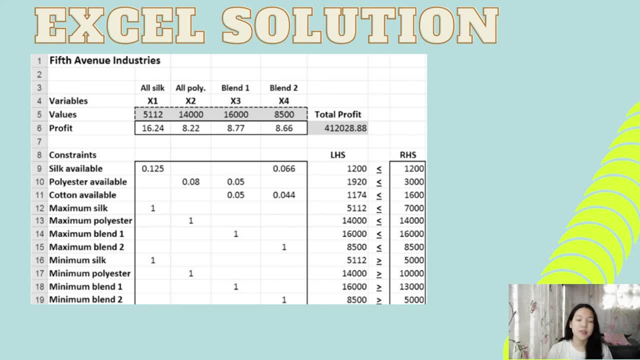 So it's just like that, guys: You have to input the data and then the Excel will solve this for you. how much is your total profit? So the result here is actually $430.. So that's it. It's actually $412,028.80.. 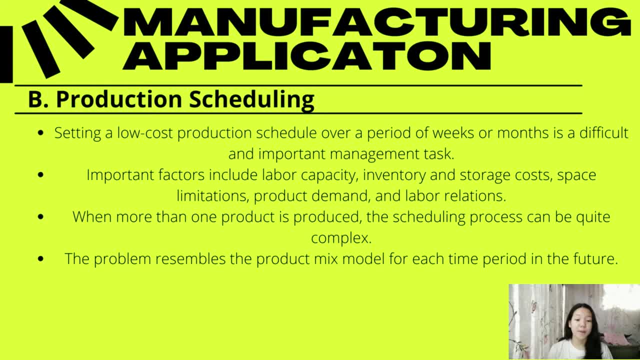 So that's a good result. Okay, moving on to the second manufacturing application, We have the production scheduling In most factories. establishing a low-cost production schedule over a period of weeks or months is challenging and critical management risk. A variety of elements must be taken into consideration by the production manager, including labor. 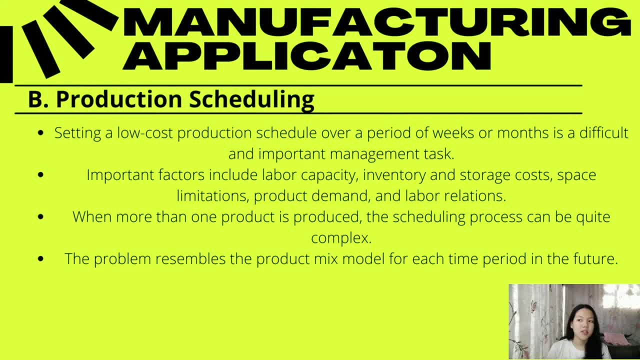 capacity, inventory and storage costs, space limits, product demand and worker relations, Given that most businesses manufacture more than one product. Yes, businesses manufacture more than one product And the scheduling procedure is frequently fairly complicated. For the most part, the problem is analogous to the product mix model for each period of 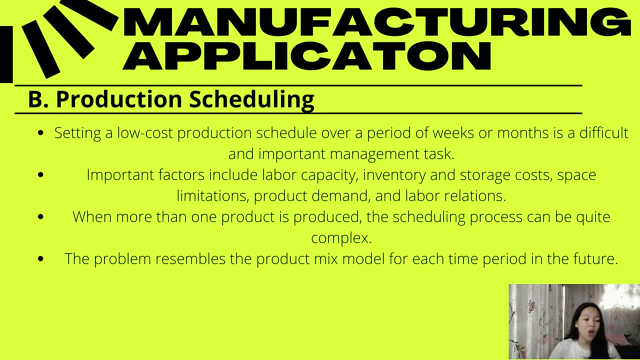 the future. The goal is either to maximize the profit or to reduce the overall cost of the carrying out of the task, including the production and inventory. So that will be discussed in the example later And as much as possible Due to the fact that the production is very complicated. 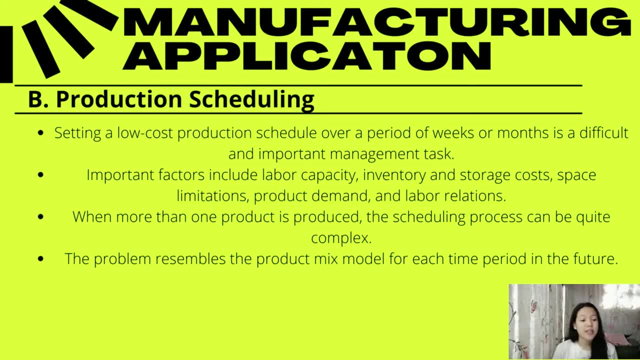 The production is very complicated. The production is very complicated. The production scheduling is a problem that needs to be solved on a regular basis. The linear programming is capable of providing a solution. When the target, function and restrictions for a firm have been defined, the inputs may. 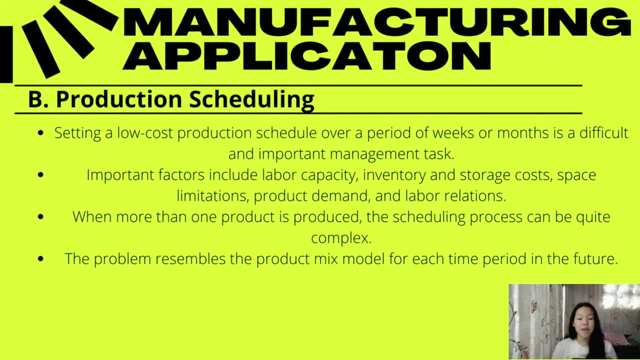 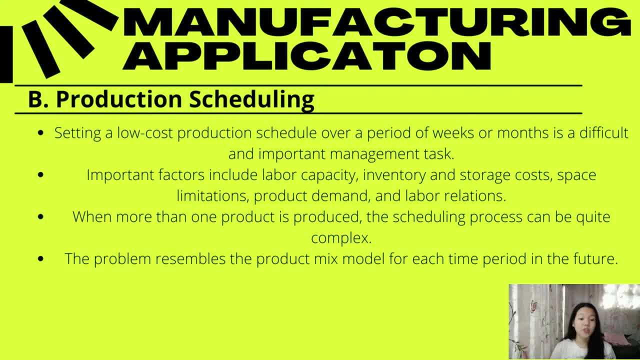 And they are more or less analyzeable in the same way. So in other words, there are clever way to to change the prices of each product. I hope few of you understand the companies that introduced as the main purpose they announced the لَقَل ڈ Kämp, and they also mention highway line. nowadays, which? 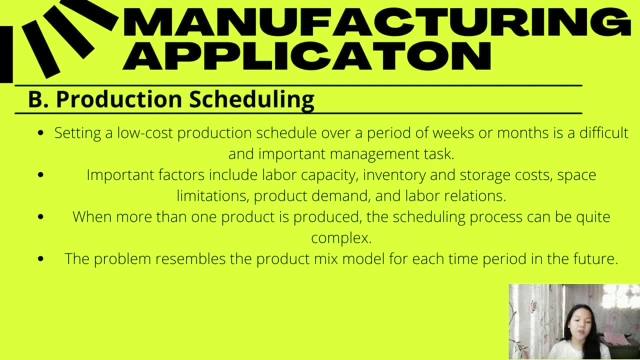 copyright like a Mediterraneanigo power graver, and they are mostly building interーン, And the proper ingredients must be present in the production facility in order for the facility to generate the items assigned to it, both for procuring and delivering components to appropriate facilities, as well as for the transporting of the final goods to the retailers. 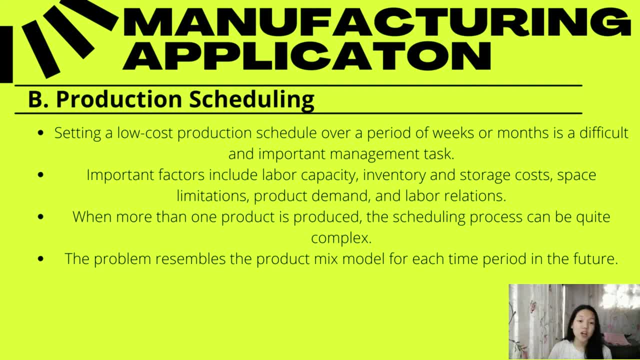 Transportation costs must be taken into consideration To account for deviations from a master plan. the linear program that monitors production planning and scheduling must be updated on a regular basis- It could be daily, or once a day, or twice a day- to ensure that items remain up to the current. 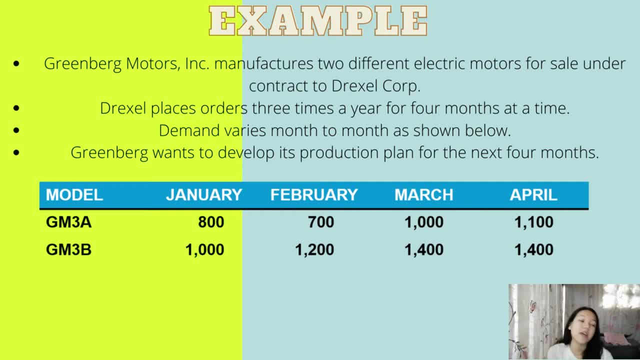 So I'll give you an example. The example here is the Green Bird Motors Incorporated, Which manufactures two different models of motors, which are the GM-3A and GM-3B, and the Drexel's order three times a year for four months at a time. 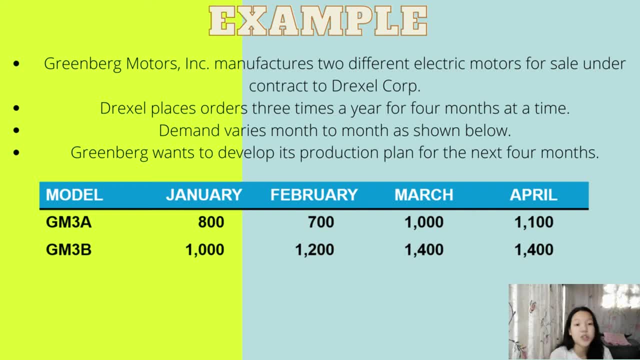 So we have here four months, from January, February, March to April. So that's four months and the demand, of course, as I said earlier, every month the demand is not really constant because it varies And the Green Bird wants to develop its production plan for the next four months. 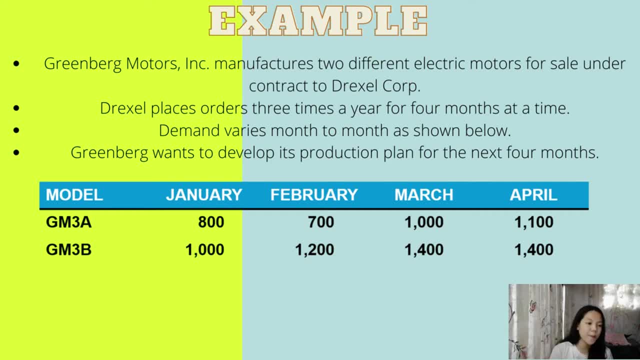 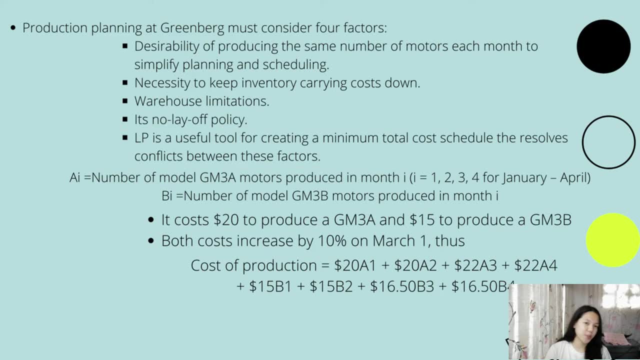 So we're going to focus for the next four months of their contract. Here we have to calculate for the cost of production. So let's start with the production. Of course, the production should consider these following factors: The desirability of producing the same number of motors each month to simplify the planning and the scheduling. 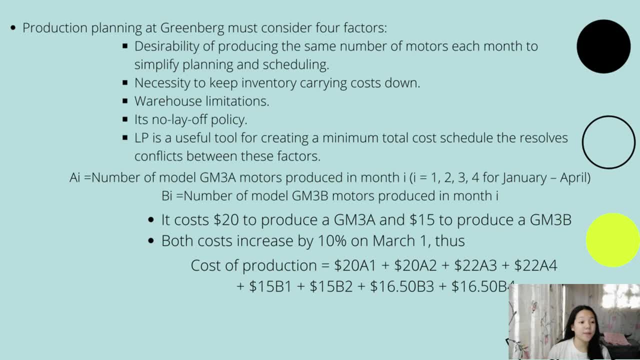 The desirability of producing the same number of motors each month to simplify the planning and the scheduling. The second one is the necessity to keep inventory carrying cost down And the warehouse limitations. It's no lay of policy and for the linear programming is a useful tool for creating a minimum total cost schedule that resolves conflicts between the factors. 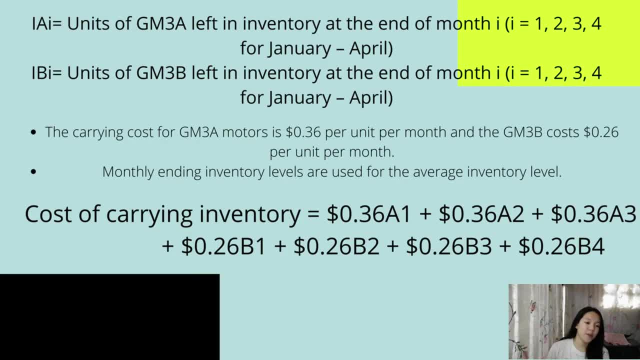 We have here variables representing the number of models, A sub i for the number of model of the GM-3A, which is the first model, and the i actually represents for the number of month, and for the bi for the second model, the number of model. gm3b model is produced in one month. here iba iba yung cost ng model per month. 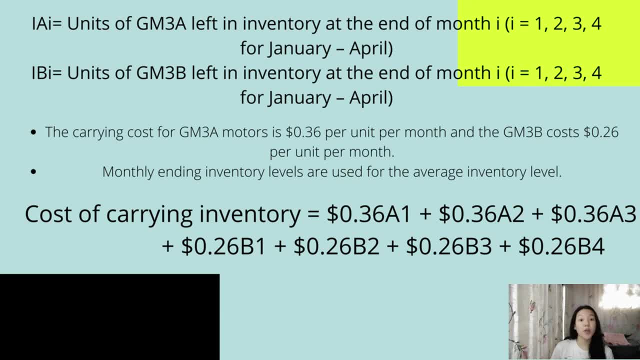 okay, it cost yung gm3a kasi nagkakosya ng twenty dollars and para mag produce ka ng, i mean to produce the first model, the gm3a, you'll be needing twenty dollars, and for the another model, the gm3 be, you'll be needing fifteen dollars, and both increase ito. 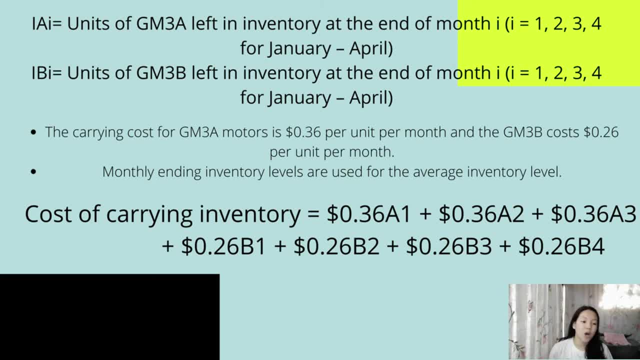 because of production is the total of the sum of the cost to produce per model. pero i noticed yung nag change yung amount niya into the third term, which is kasi the third term is the third month, which is the March. So disregard natin na hindi natin kukuno ng 10% yung from January up to February, since yung 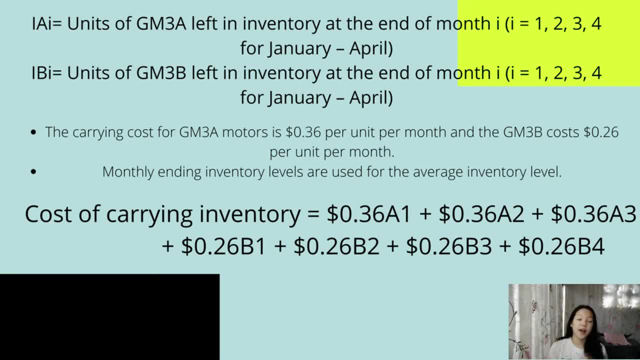 pag-increase ng 10%, na start lang siya sa March, So hanggang April na yon nag-increase siya ng 10%, So the other one will also increase in the 10%. I mean the second one, from 15 naging 16.50, kasi may 10% tayong dinagdag doon. 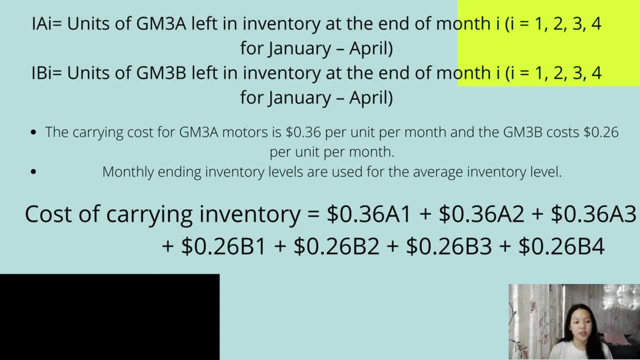 And here is ang kailangan naman natin i-solve is the inventory. I mean kuha na ng equation or ng function Represent. so here is the variable, the IA sub I, which means the units of GMT left in inventory at the end of the month. 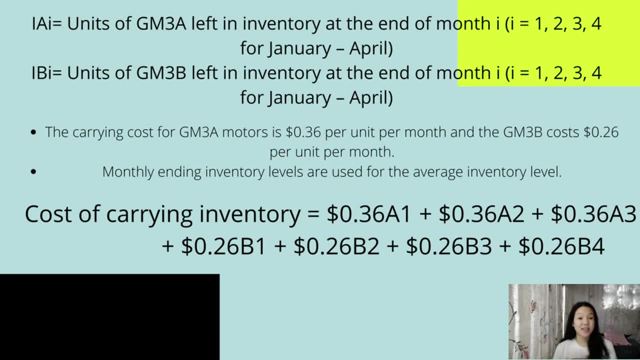 And for the IB sub I is also the same, Representing the second unit of model. Okay, meron din tayong different cost per inventory dito per model which is yung GM3A. yung first model costs $0.36 per month. 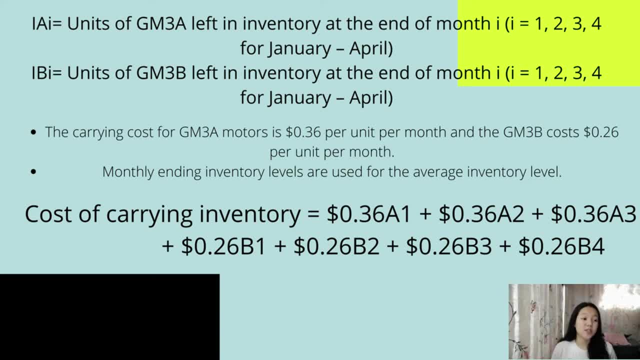 While the second model, the GM3B, costs $2.26 per unit per month And the monthly ending inventory levels are used for the average inventory level. So here is its function for the inventory And this is what we found in this slide. 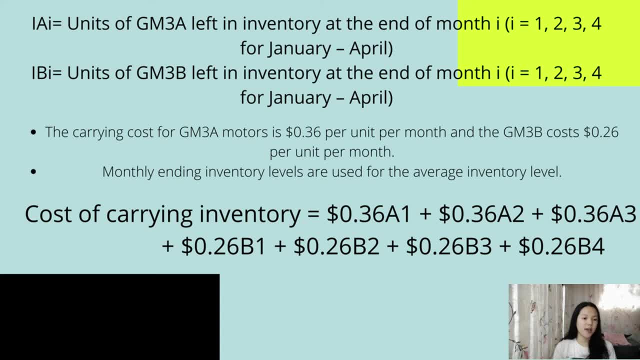 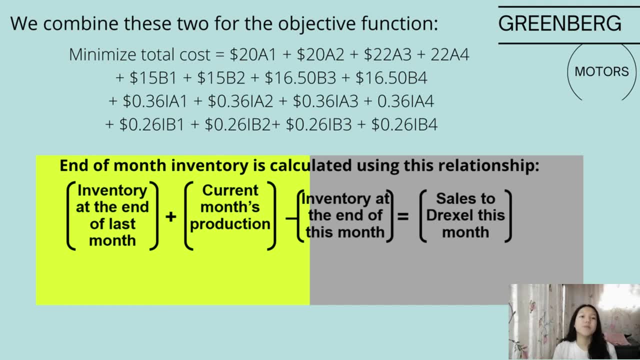 First lang din, disunod lang din yung conditions and gimit lang siya. Okay, combining those functions will be forming our objective, which is to minimize our total cost. So yun lang, yung two objectives ng inventory and production is i-combine para maka-solve tayo ng minimal- para ma-minimize natin yung total cost natin. 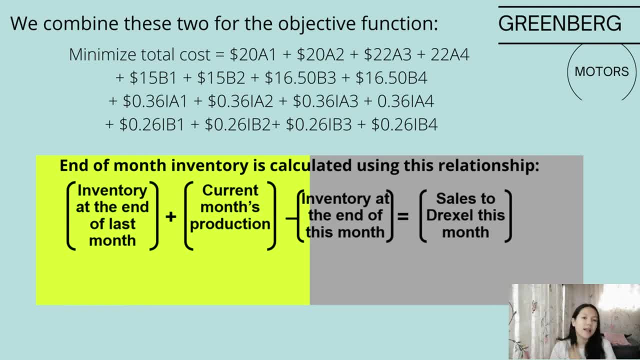 So that's how we solve for that And mamaya, sa Excel, and maybe you want to try na i-input itong data na ito for you to solve And showing here the end of the month inventory, how to be calculated. Okay, inventory at the end of the last month plus the current month's production, less than the inventory of the end of the month, is equal to sales ng Drexel ngayong month. 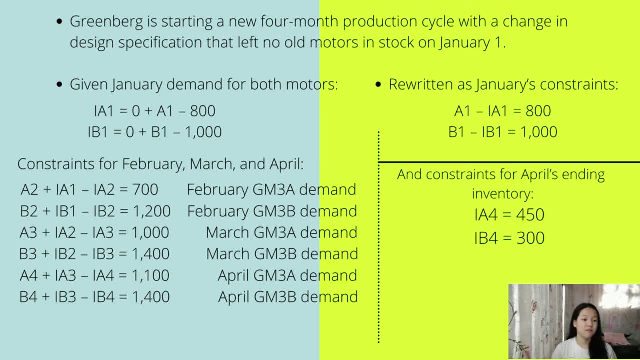 Dito may changes sa demand. Greenberg is starting a new four-month production, A new four-month production cycle with a change in design Specification to the left. no old motors in stock on January. So January na naman yung pakikialaman natin dito. 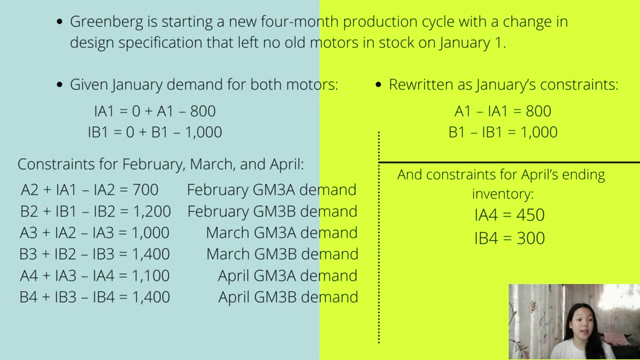 Since yung demand ng January is from two different models is 800 to 1,000. We're going to rewrite it as A sub 1 less than inventory na I. A sub 1 is equal to 800.. And then for the next model, is the B sub 1 less than the I B sub 1 equal to 1,000. 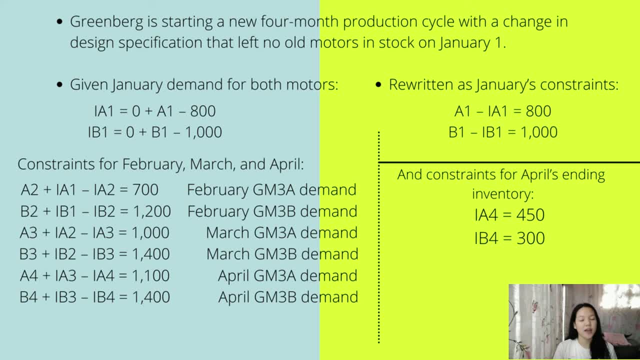 Of course, for the proceeding month, din tayong constraint doon which is given here Ayan, And the other constraint for the ending inventory ng April is I A sub 4 is equal to 450.. And for the second model, the I B sub 4 is 300. 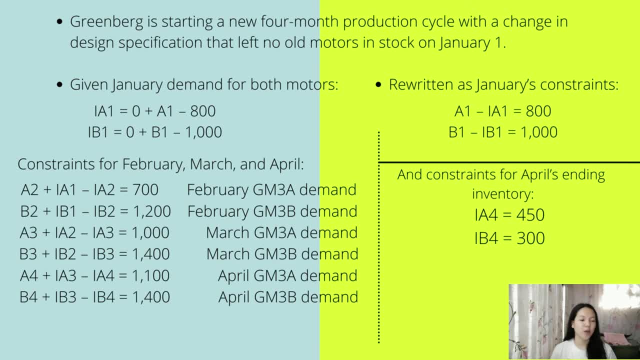 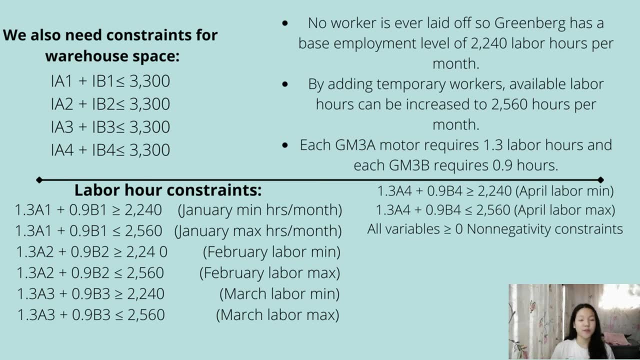 Ayan Yung mga makahalagang information for our solving to the Excel, And Hindi lang yun ang dapat gina-consider, because we have to consider for our labor hours And, of course, gaya ng sinabing kanina, is yung warehouse space. 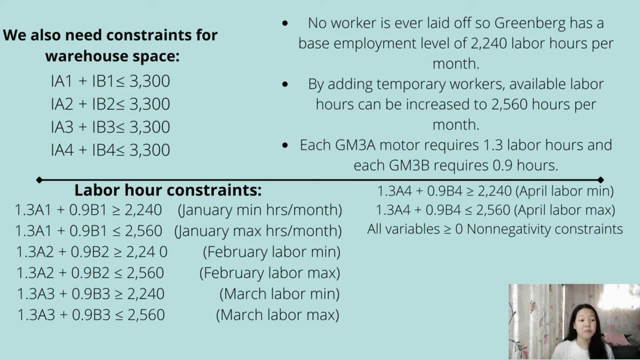 And no workers is ever laid off. So the Greenberg has a base employment of level of 2,200 labor hours per month And by adding the temporary workers, yung available labor hours can be increased to 2,560 hours per month. 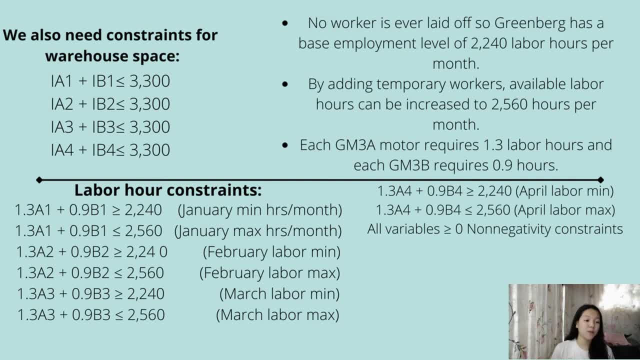 And each GM3A Yung first model model requires 1.3 labor hours And each GM3B- second model requires 0.9 hours. So here is its constraints written below. So medyo complex sya kasi marami syang constraint na hinahanap. 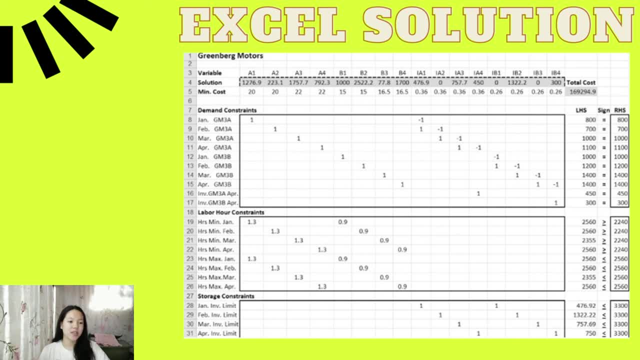 And here is its Excel solution. So makikita nyo na tatlo yung constraints, na I mean tatlong groups ng constraint, yung Yung they provide, And here is its solution or here is its answers. Okay, for the January units produced here. 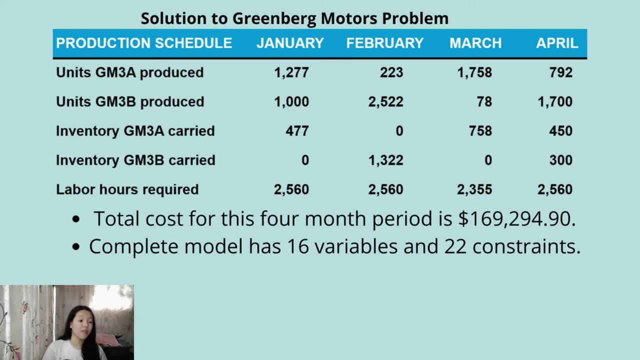 For the GM3A is 1,277 and so on and so forth. And of course yung units din ng GM3B, ng the January, is 1,000 and so on and so forth, And yung inventory, ito din yung result. And of course, to the labor hours required From January to April. nag-vary din, So iba iba yung result per month, Since walang constant dito, And for the total cost for this 4 months period is $169,949.90.. 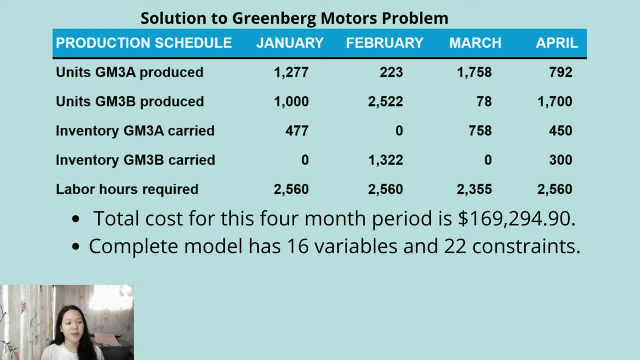 And actually yung complete model mayroon 16 variables And it composed of 22 constraints also, So masyadong marami. So that's how it's. that's how complicated it should. I mean that's how complicated it is. 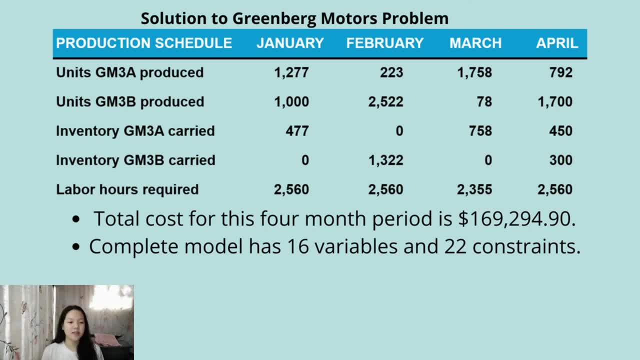 Pero linear programming could make it easier naman, Kasi. you just have to identify your data, So you just have to input your data. So then, Ayan na Excel solver will do it for you, And for the next topic we'll have another reporter. 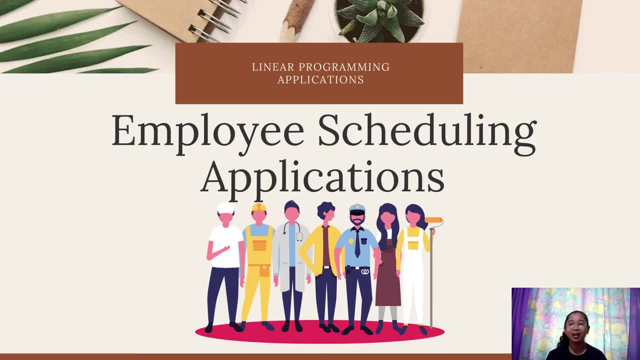 Thank you. Good morning everyone. The next topic is about employee scheduling applications. Here we will learn about these applications in the real world And know how to utilize it in the excel solver. Specifically, I'm going to discuss or introduce to you the use of linear programming. 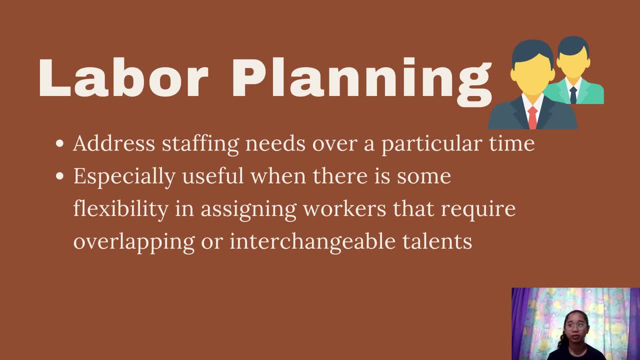 To help businesses deal with a shortage of workers. Labor planning is a schedule which is developed or set. It is an act of balancing in a process to make sure that the persons with appropriate skills are where they are needed at the moment, Ensuring they have all the necessary skills and abilities. 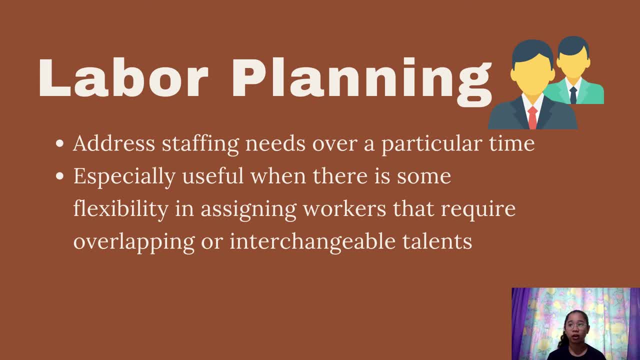 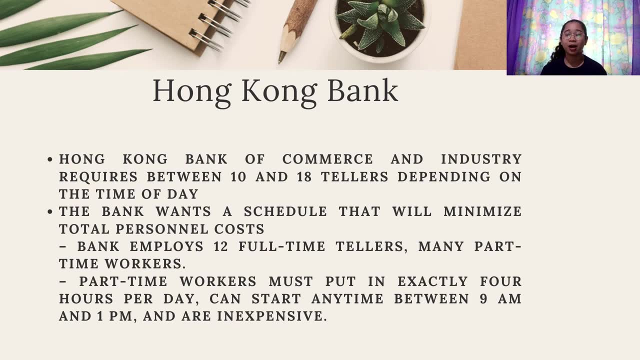 This will also help reduce the overall cost for the organization. Many banks employ the LP method, which is used for handling labor scheduling. The Hong Kong Bank, for example. Tellers at the Hong Kong Bank of Commerce and Industry are hired according to the hours of the day. 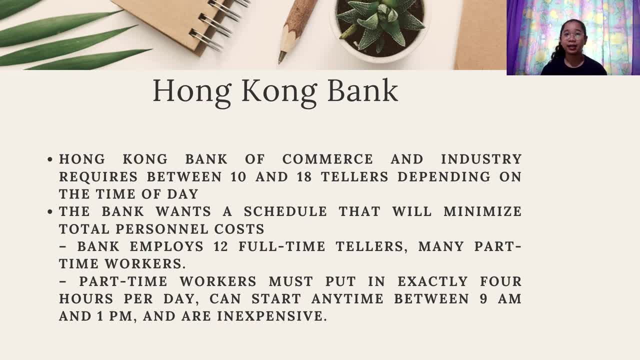 To keep labor expenses down, the bank allocated tellers to positions at a certain time of day. Even though it has a 12 person staff, many workers are still on the bank's part time roster. A part time employee is expected to be present for at least 4 hours per day. 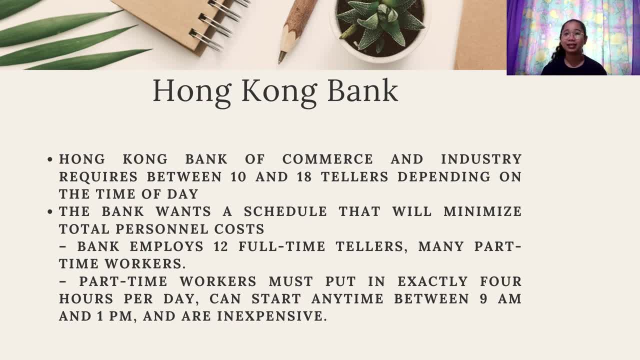 But can begin as early as 9 am and as late as 1 pm. Part time workers have a reasonably low cost to the company since they do not receive retirement or lunch benefits. Full time workers are granted an hour for lunch and are on the job from 9 am to 5 pm. 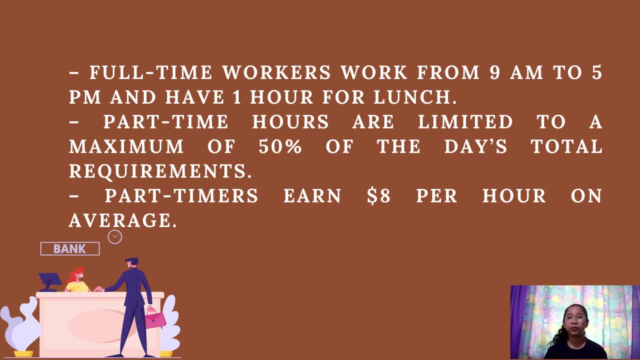 At 11 am, half of the full time workers eats while the other half works. Full time workers contribute to the company. They get 35 hours of productive time per week. The bank implements a policy through which part time work hours are limited to the maximum of 50% of the total required work hours per day. 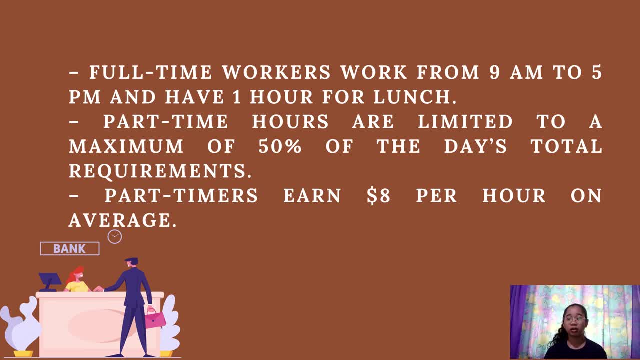 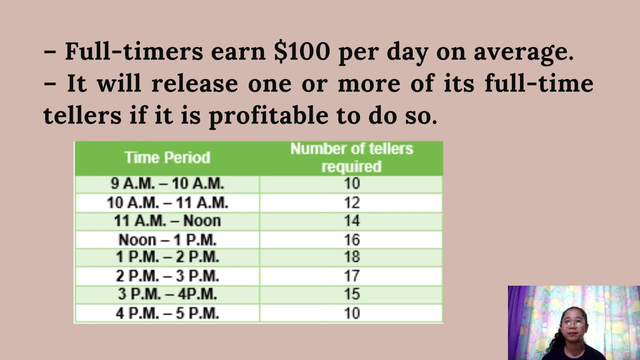 On the average, part time workers make $8 per hour or $32 per day. Full time employees receive an average of $100 a day in compensation and benefits. To minimize total labor costs, the bank wants to implement a scheduling method that can be implemented on a regular basis. 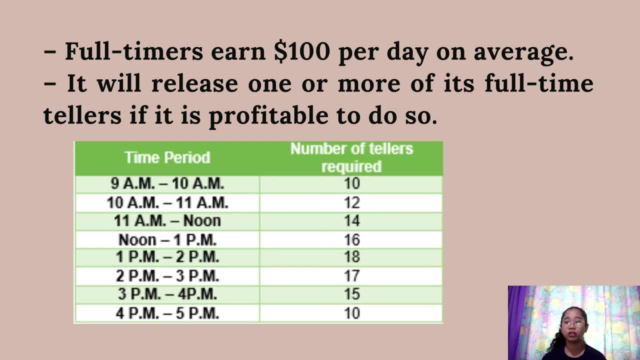 When it's in the interest of the company to do so. like Profitable, it will release some of its full time tellers. The table shows the number of personnel that the bank needs in a various periods of the day when it is open. 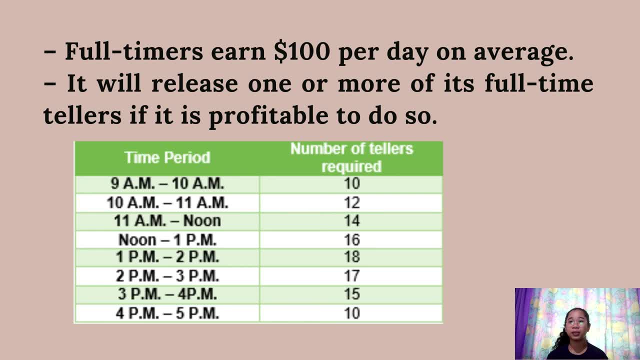 It's most obvious that during lunch, between 12 and 2 pm, is the busiest time of the day. A limitation is enforced every hour of the day and it states that at least the minimum number of employees are required during that time. Therefore, there are 8 of these constraints which are required. 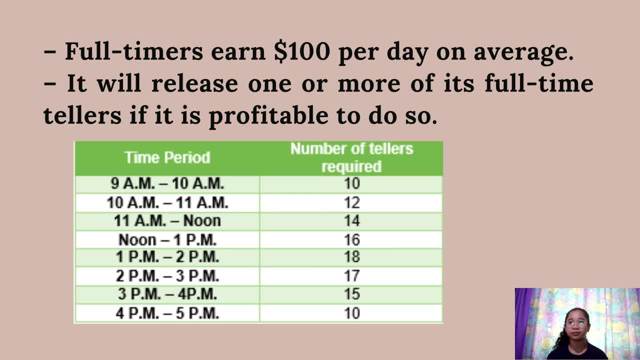 These constraints are from 9 am to 5 pm. We will also impose a restriction on the overall number of full time workers, and this cap will be 12.. The last constraint will specify the number of part time hours. that should not exceed 50% of the total hours. 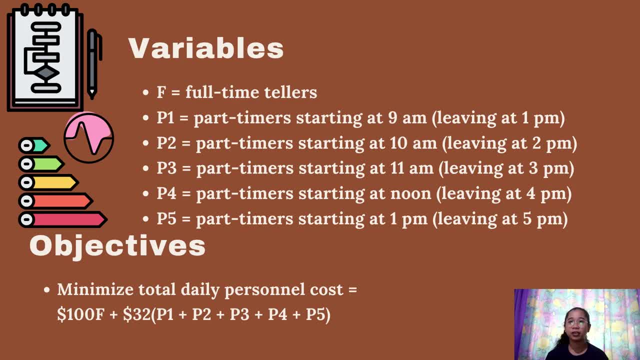 Here are the viables that we can use to achieve the goal or objective, which is to minimize cost of daily personnel. Let F as the full time tellers, P sub 1 as a part timer. P sub 2 as a part timer starting at 9 am. 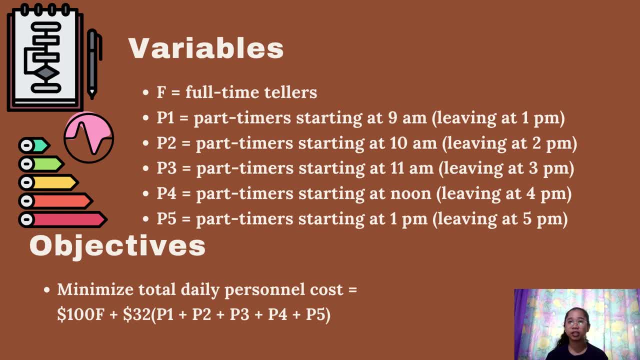 P sub 2 as a part timer starting at 10 am, P sub 3 as a part timer starting at 11 am, P sub 4 as a part timer starting at noon and P sub 5 as a part timer starting at 1 pm. 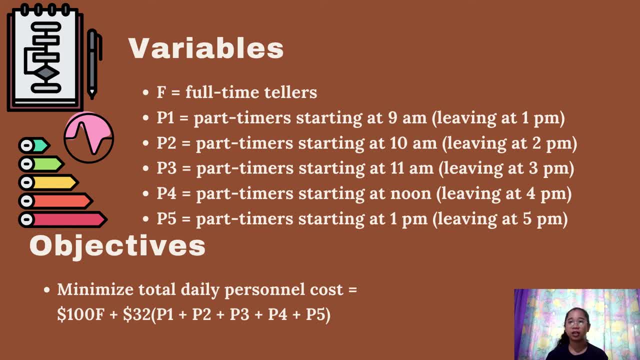 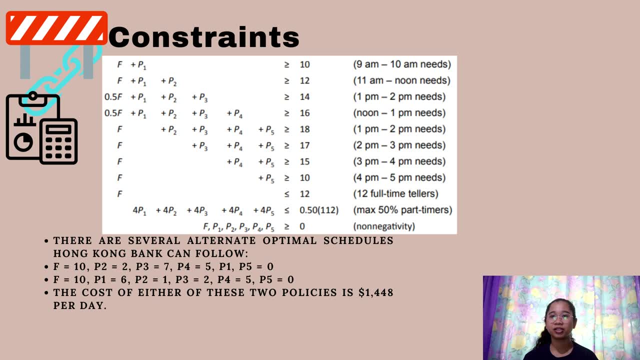 The objective is to minimize the total daily personnel cost and to get this, the salary of full time and part time workers will be added and multiplied. These constraints are scheduled of how many personnel, either full time workers or part time workers, should work within an hour. 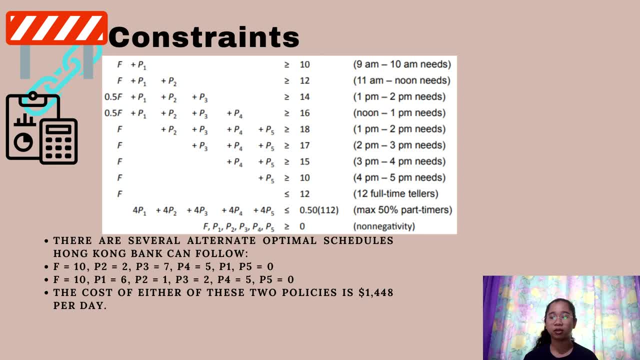 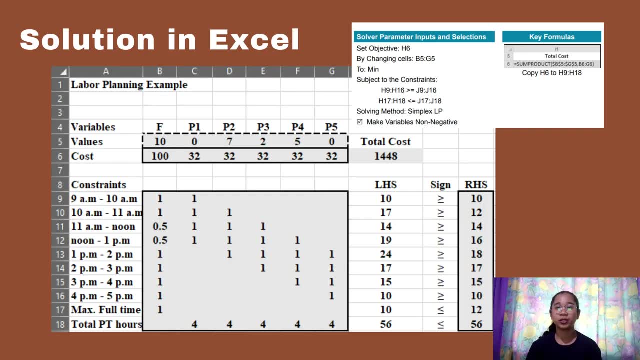 There are two optimal schedules for Hong Kong bank to follow, But as for this scenario, we will use the first sketch as an example. Here is the example solution in excel for labor planning schedule. As what I have said earlier, the variables, these are the workers or personnel which work full time and part time. 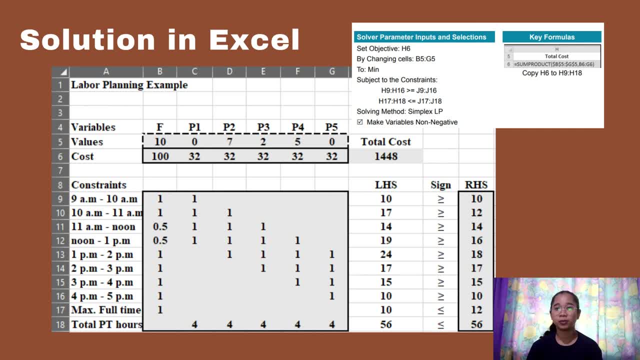 Then these values are one of the optimal schedules which is given by using the excel solver. The cost or the salary of the workers for a day: $100 for the full time, then $32 for those who work part time. The number one means that all workers work at that time of the day. 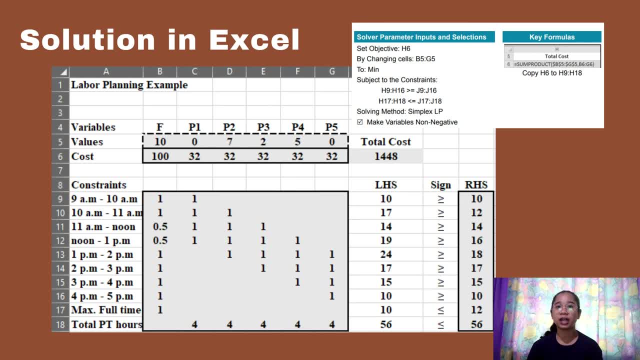 We can say that 0.5 is that only half of the workers work at a particular time while the other half are having their lunch. The computation using the excel solver are shown from the previous reporter, Though it was a different example yet the process of how did we ended up with the amount of values. 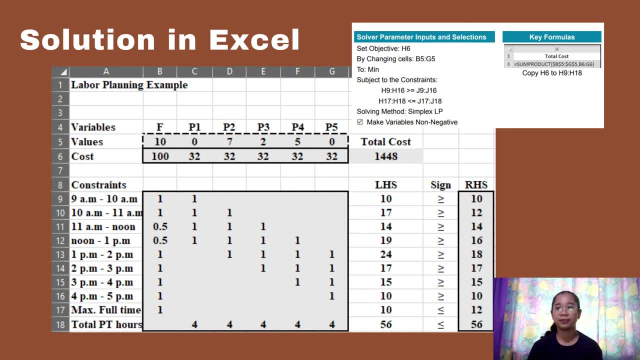 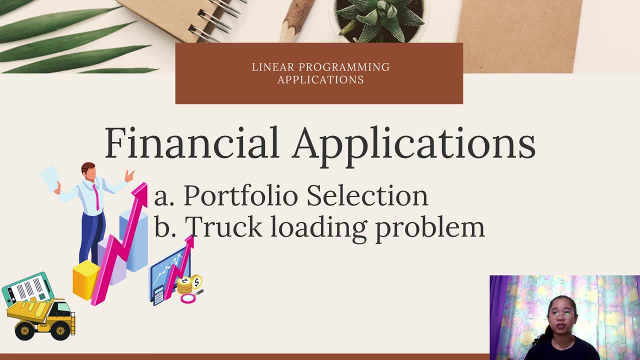 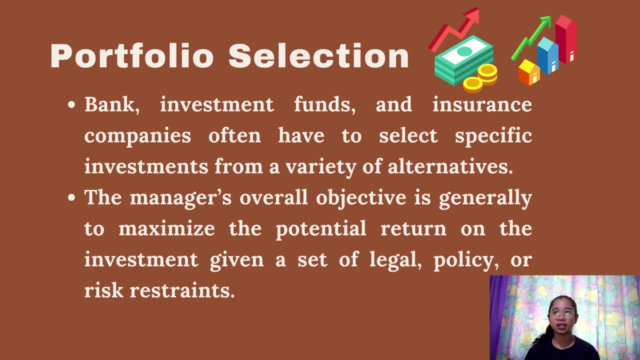 LHS and the objective or the total cost is the same. The next topic will be about the financial applications, And under these are the portfolio selection and the truck loading problem. But first let us discuss about the portfolio selection. Portfolio selection is a process by which one chooses the securities, derivatives and other assets to include in a portfolio. 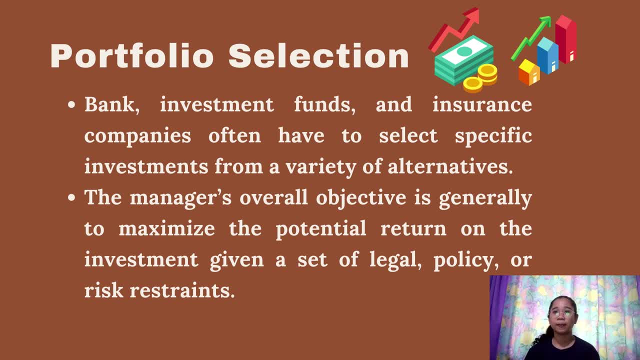 In making security selections, one considers the risk, the return, the ethical implications and other factors affecting both of the individual securities and the portfolio as a whole. In portfolio selection, one's objective is to maximize the potential return on investment from a variety of alternatives. 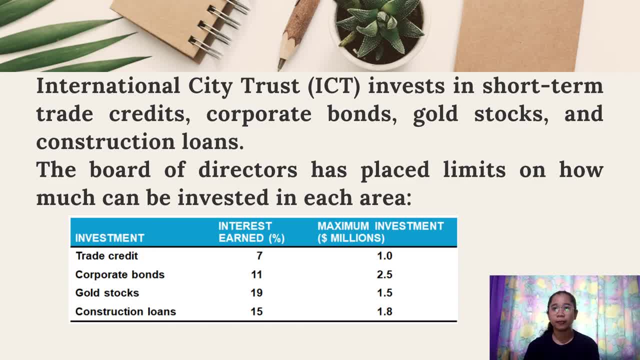 For example, the International City Trust. You want to invest in four different fields, which are the trade credit, corporate bonds, gold stocks and construction loans. The table shows how much each field is worth, How much each field has its rate of return. 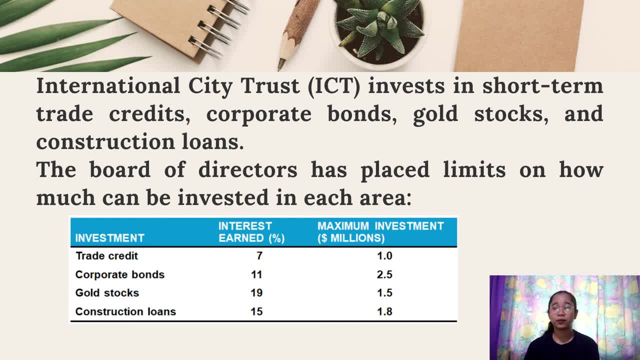 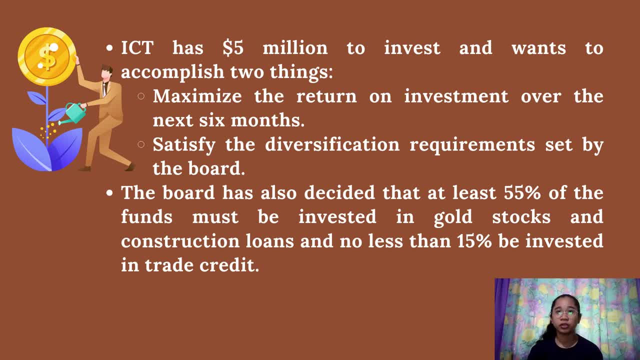 7% for the trade credit, 11% for the corporate bonds, 19% for the gold stocks and 15% for the construction loans. The ICT wants to accomplish two things by investing $5 million. First is to maximize the return on investment for the next six months. 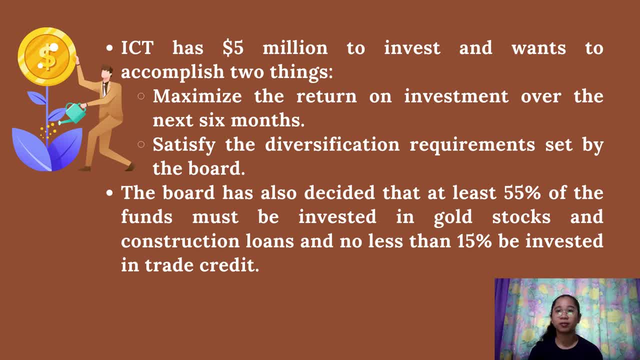 And then satisfy diversification requirements set by the board. Diversification is a process which it allocates its capital or invested from the different fields to reduce risk. Moreover, the funds invested in gold stocks and construction loans should be at least 55% or higher its total budget. 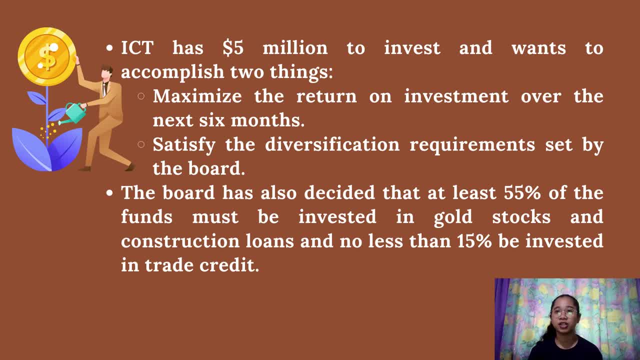 In addition, no less than 15% of the budget should be invested in trade credit. However, the ICT only has a $5 million budget and the company set a maximum investment for each field based from the table shown previously. Yet the company wants to maximize the return on investment. 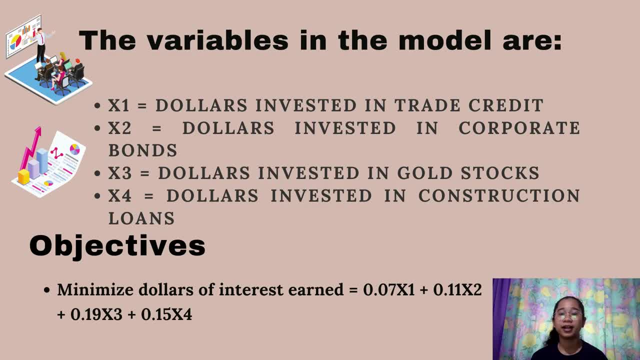 With these investment conditions, Here are the viables that will be used, which are: X1- as the dollars invested in trade credit. X2- as the dollars invested in corporate bonds. X3- as the dollars invested in gold stocks. And X4- as the dollars invested in construction loans. 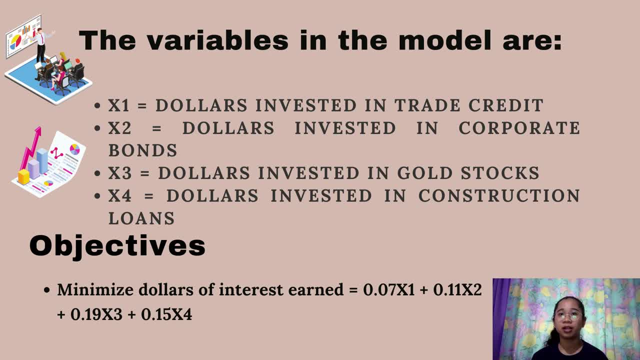 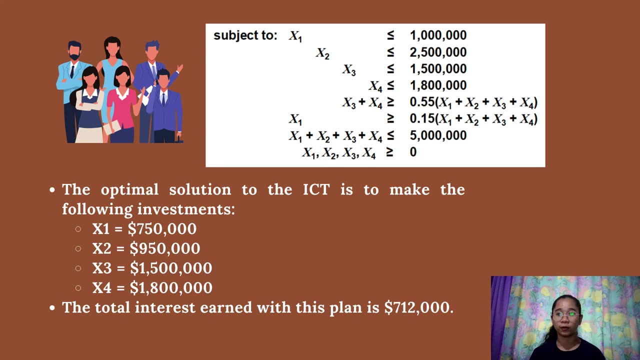 The objective of ICT is to minimize dollars of interest earned with the help of the equation, which is interest from the different fields multiplied to invested capital and by adding its product. Here are the constraints that will be used in solving the equation by using the Excel solver. 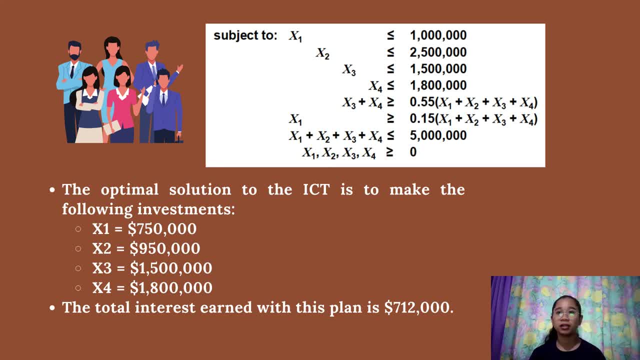 The optimal solution to the ICT is to make the following investments: The X1,: they will invest an amount of $750,000.. For the X2, an amount of $950,000.. For the X3, an amount of $1.5 million. 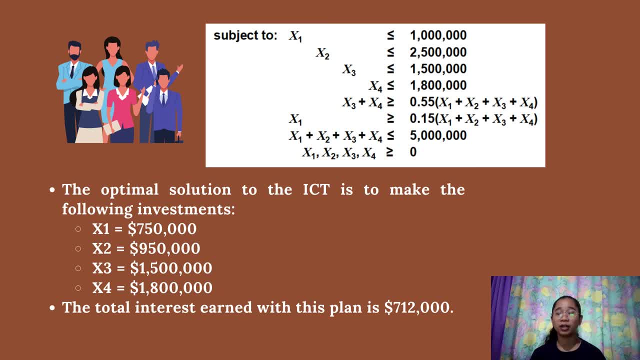 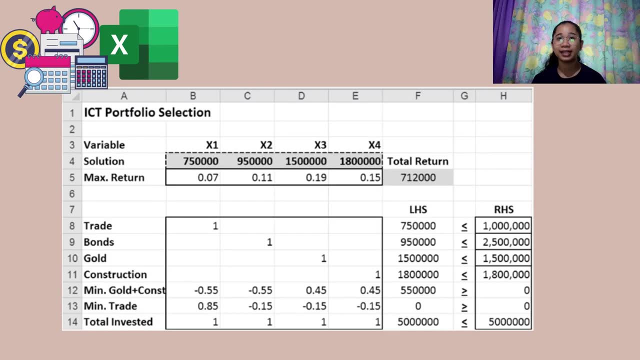 And for the X4, an amount of $1.8 million. The total interest earned with this plan is $712,000.. In this table, the total cost LHS and the solution will be given by using the Excel solver. 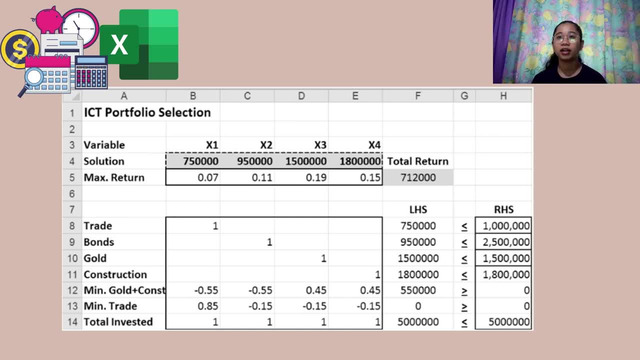 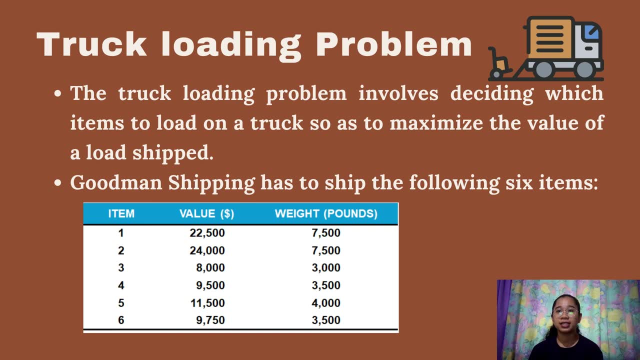 The max return is from the objectives and the RHS is from the constraint which the variables or the problem is subject to. The truck loading problem involves deciding which items to load on a truck so as to maximize the value of a load ship. The truck loading problem is about selecting the item which is most profitable that you can transport on a truck. 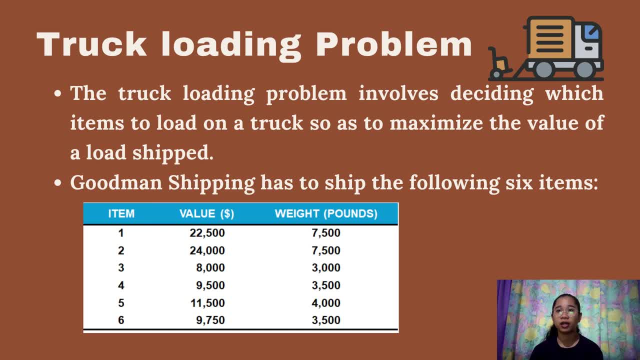 Since the truck has a limit of how much items should be loaded based from its weight, truck hauling loads exceeding gross vehicle weight ratings can lead to equipment and brake failures, as well as increased stopping distances. The table below shows the items which needs to be shipped by the Goodman Shipping, with its value and weight. 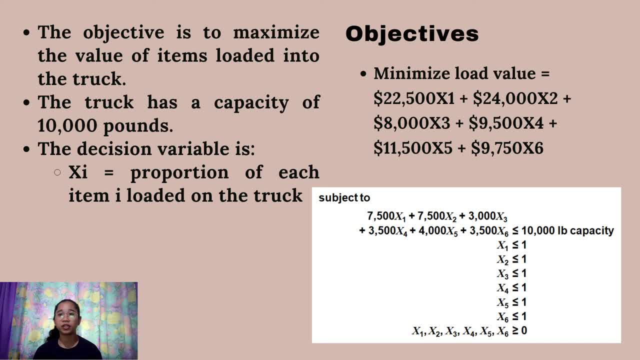 The goal of this problem is to maximize the value load in the truck without exceeding the truck's weight, but also minimizing the load or items in a truck which should be less than or equal to 10,000 pounds. The decision variable is the X sub i or the proportion of each item loaded on a truck. 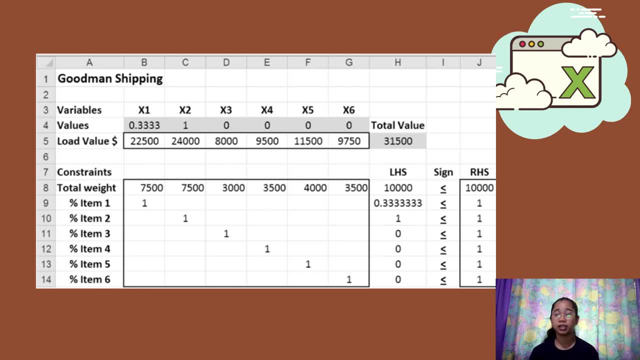 This slide shows the generated answer or solution by using the Excel solver. The table shows how much the total value should be shipped, which is $31,500.. The Goodman Shipping problem raises an interesting issue. The solution calls for one-third of item 1 to be loaded on a truck. 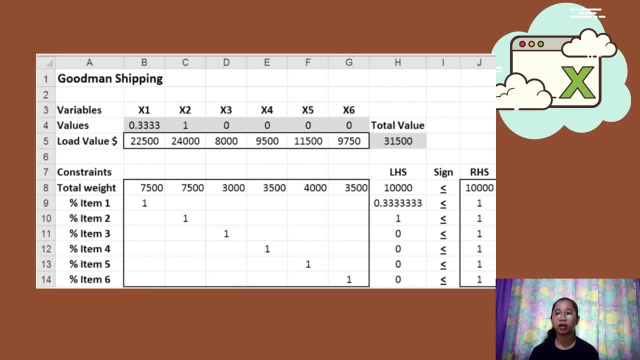 Rounding down leaves unused capacity on a truck and results in a value of $24,000.. Rounding up is not possible since this would exceed the capacity of the truck Using integer programming, in which a solution is required to contain only integers. 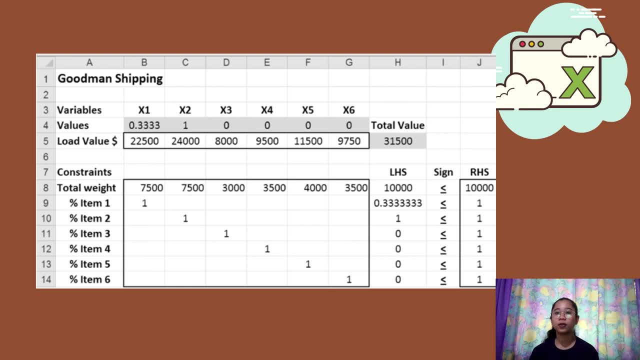 the solution is to load one unit per truck. The solution is to load one unit of items 3,, 4, and 6 for a value of $27,250.. And this ends my report about the employee scheduling applications and financial applications. 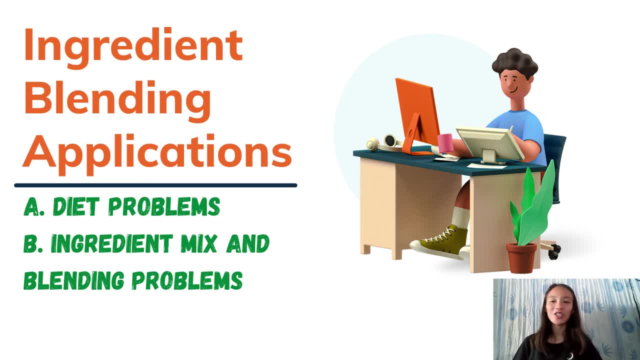 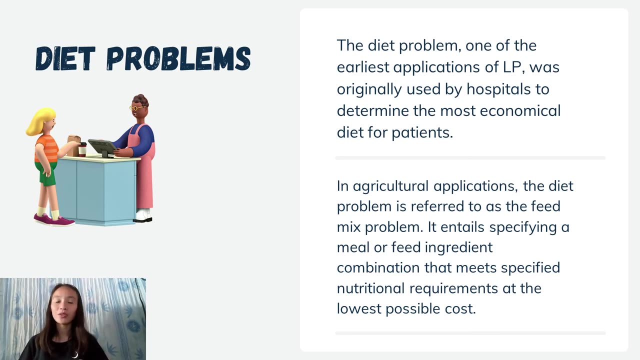 So good morning everyone. Our next topic is about the ingredient blending application, And under this application we have two topics: the diet problem and the ingredient mix and blending problems. So first let's talk about the diet problem. So diet problem is one of the earliest applications of linear programming. 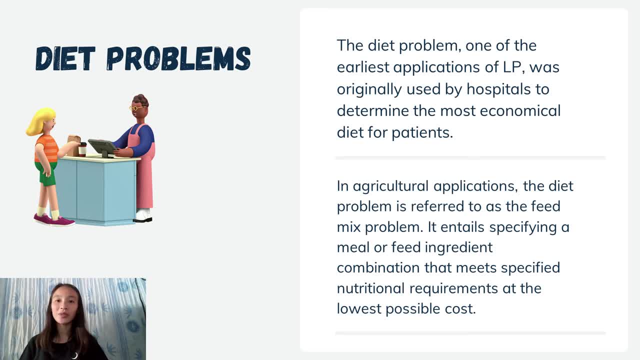 And it was originally used by hospitals to determine the most economical diet for their patients. It is known in the agricultural applications as the feed-mix problem. The diet problem involves specifying a food or feed-ingredient combination that satisfy the stated nutritional requirements at the minimum cost level. 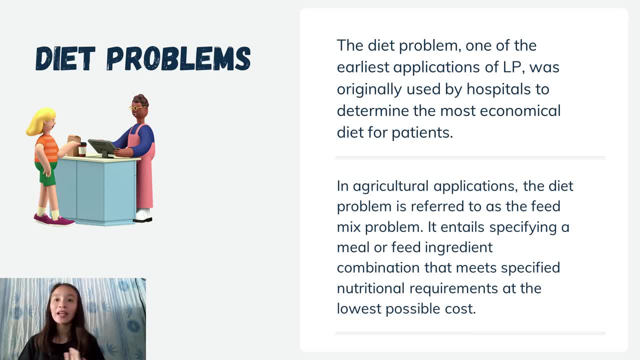 So the goal of the diet problem is to select a set of food that will satisfy a set of daily nutritional requirements at a minimum cost. The problem is formulated as a linear program, where the objective is to minimize the cost and the constraints are to satisfy the specified nutritional requirements. 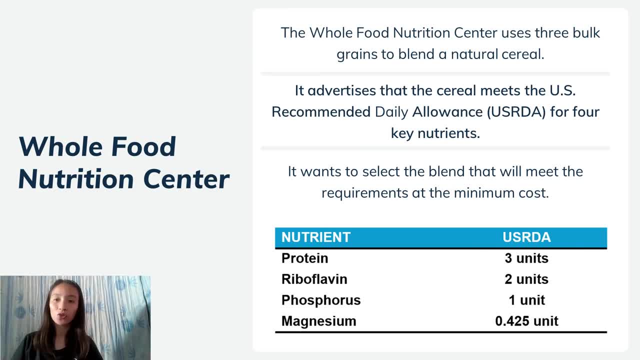 So for this application let's use the Whole Food Nutrition Center as our example. So the Whole Food Nutrition Center uses three bulk of grain to blend a natural cereal. It advertises that the cereal meets the US recommended daily allowance for the four key nutrients. 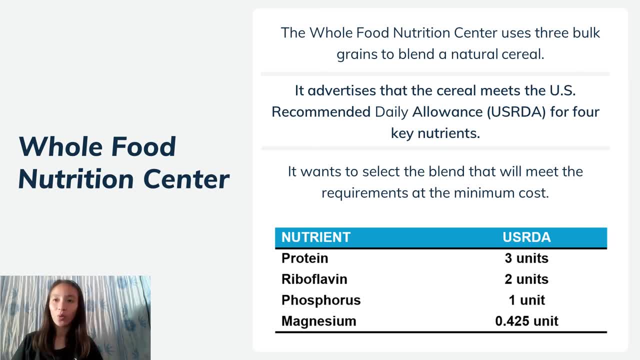 It wants to select a blend that will meet the requirements at the minimum cost. So the table below shows the four key nutrients their cereal contains, and these are protein, riboflavin, phosphorus and magnesium. The other column of the table shows the amount of nutrients. 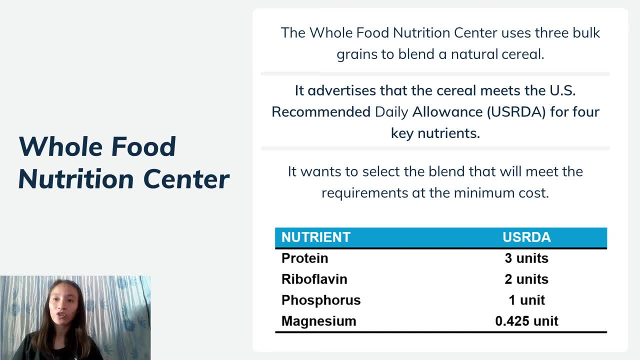 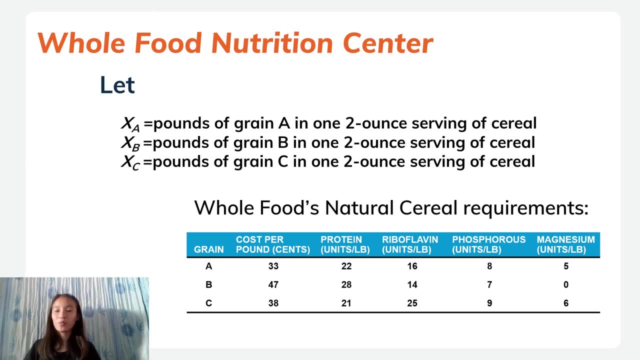 recommended by the US RDA for each two-ounce serving of their cereal. In modeling this as a linear program, the objective is to minimize the cost. There will be four constraints: one each for protein, riboflavin, phosphorus and magnesium. 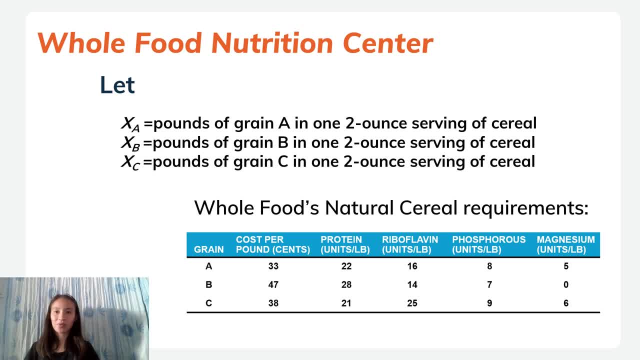 showing the number of units for the minimum amount specified. Since these requirements are for each two-ounce serving the last constraint, must say that the total amount of the grains used will be 0.125 pounds In order to calculate the total cost. 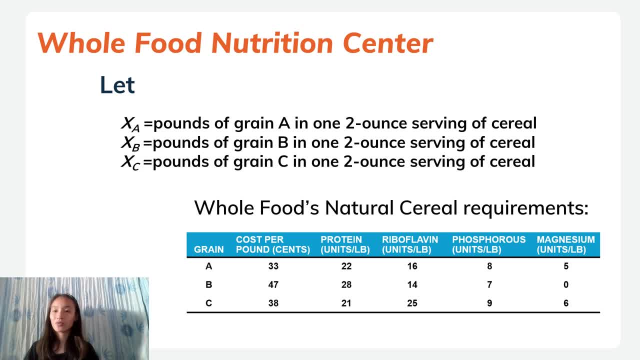 we must know the number of pounds of the grains used in one serving of the cereal. Also, the numbers in the table below are expressed in units per pound of grains, so defining the variables as the number of pounds of the grains makes it easier to calculate the amounts of protein, riboflavin, phosphorus and magnesium. 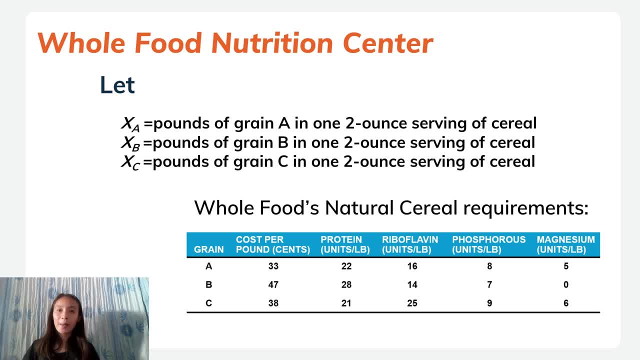 For the variable, we let X of A be pounds of grain A in one two-ounce serving of cereal, X of B be pounds of grain B in one two-ounce serving of cereal and X of C be pounds of grain C in one two-ounce serving of cereal. 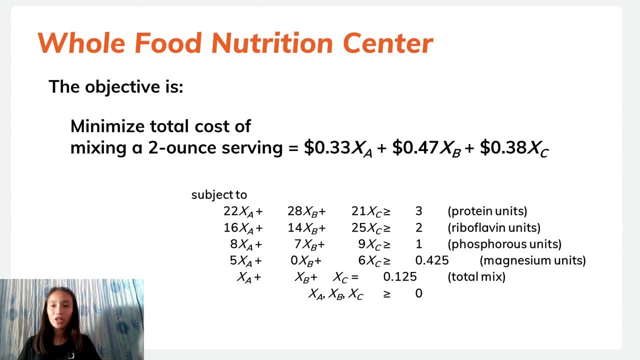 The objective for this example is to minimize the cost of mixing a two-ounce serving, which is equal to the sum of 0.33 dollars X of A plus 0.47 dollars X of B plus 0.38 dollars X of C. 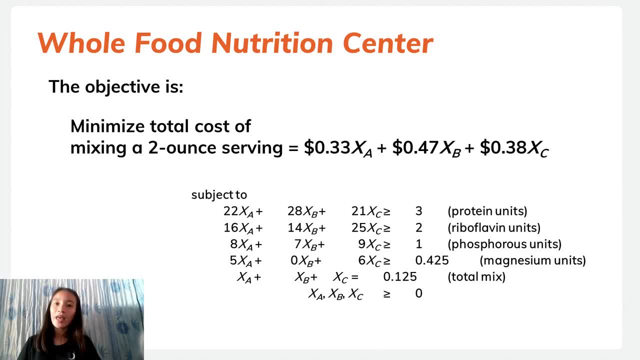 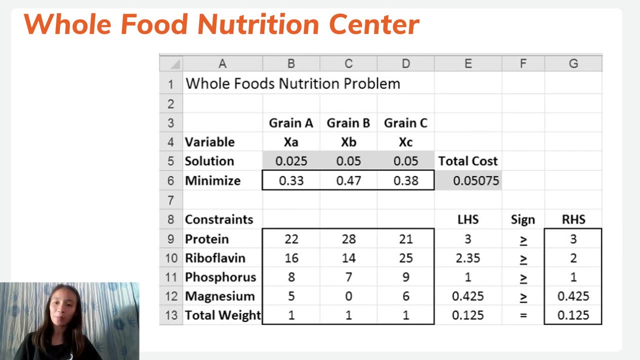 which is subject to the constraints below And, as I've mentioned earlier, we have constraints for each of the nutrients and the last constraint is about the total amount of grains used. The picture illustrates the solution for the example using the Excel solver. It shows the variable, which are the 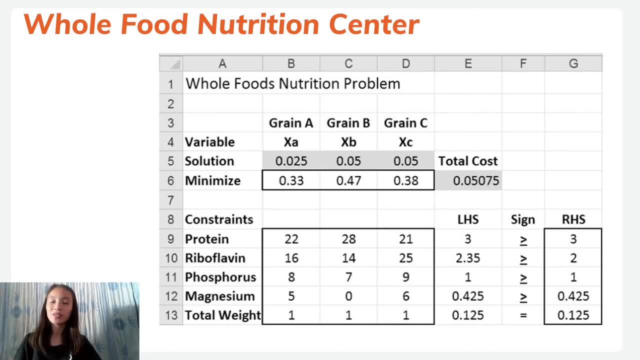 X of A, X of B and X of C. that represents the pounds of grain A, grain B and grain C, the objective, the constraint and the LHS and the RHS. The solution for this requires mixing together 0.025 pounds of grain A. 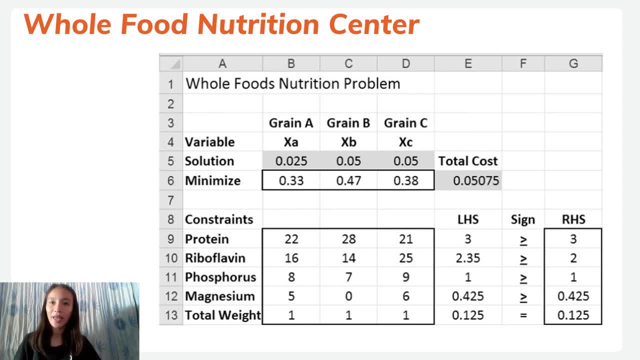 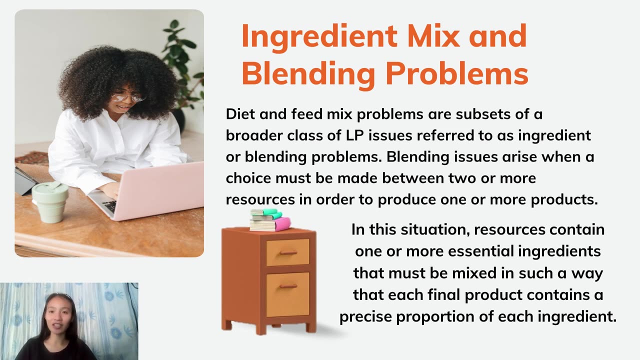 0.050 pounds of grain B and 0.050 pounds of grain C, And the total cost per serving is equals to 0.05 dollars. So our second topic under the ingredient blending application is the ingredient mix and blending problems. 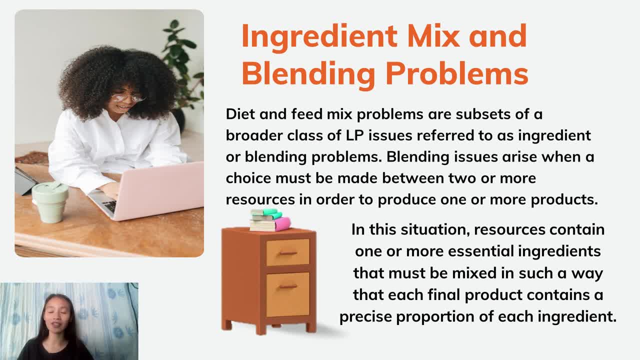 So diet and feed mix problem are subsets of a broader class of linear programming issues, referred to as ingredient or blending problems. Blending problems arises when a choice must be made between two or more resources in order to produce one or more products. So in this situation, 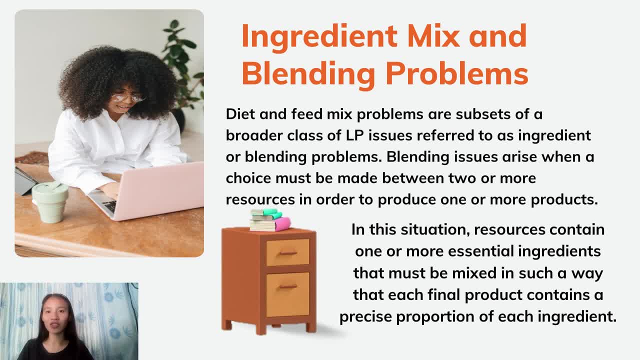 resources contain one or more essential ingredients that must be mixed in such a way that each final product contains a precise portion of each ingredient. So in the ingredient mix and blending problem, it is about the mixing of important ingredients in order to form a final product. 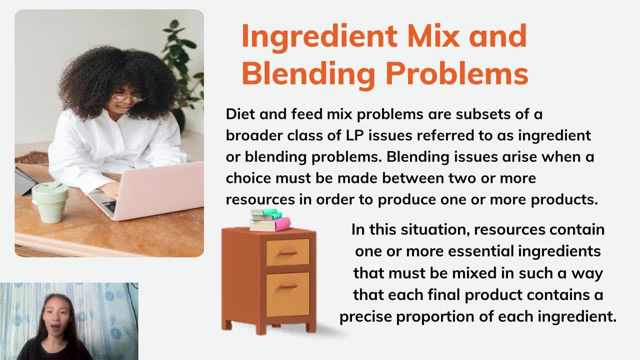 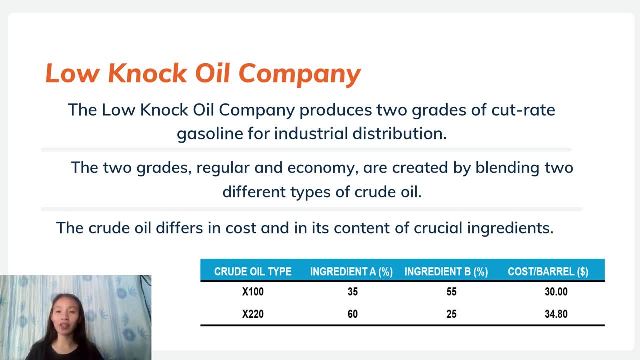 Then the product contains a specified amount of each ingredient. So our example for this problem deals with an application of linear programming in the petroleum industry: The blending of crude oils to produce refinable gasoline. So the Lonac Oil Company produces two grades of cut-rate gasoline. 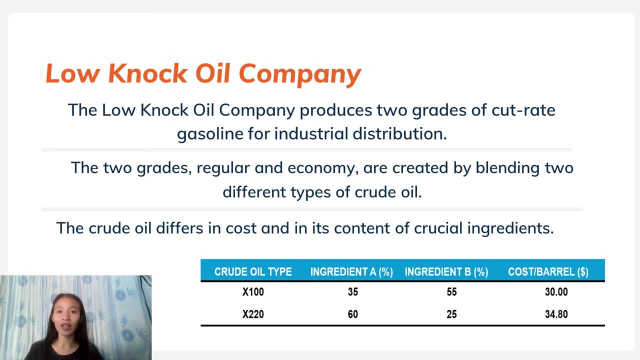 for industrial distribution. The two grades- regular and economy, are created by blending two different types of crude oil. The crude oil differs in the cost and its content of crucial ingredients, And the table below indicates the two types of crude oil. The percentage of crucial ingredients found in each crude oil. 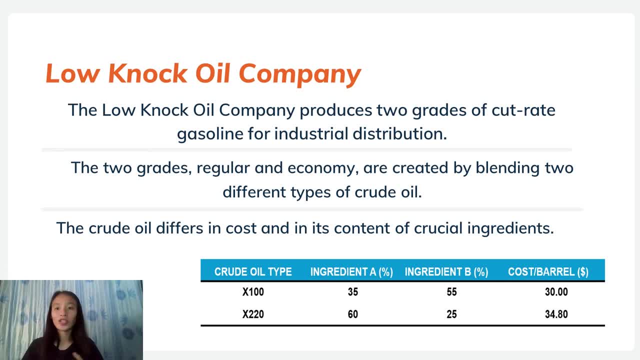 and the cost per barrel for each. Weekly demand for the regular grade of Lonac gasoline is at least 25,000 barrels And the demand for the economy is at least 32,000 barrels per week. At least 45% of each barrel of regular must be ingredient A. 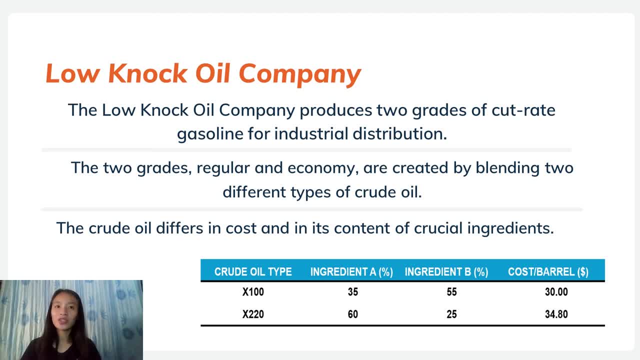 And at most 50% of each barrel of economy should contain ingredient B. The Lonac management must decide how many barrels of each type of crude oil to buy each week for blending to satisfy demand at a minimum cost. In modeling this as a linear program, 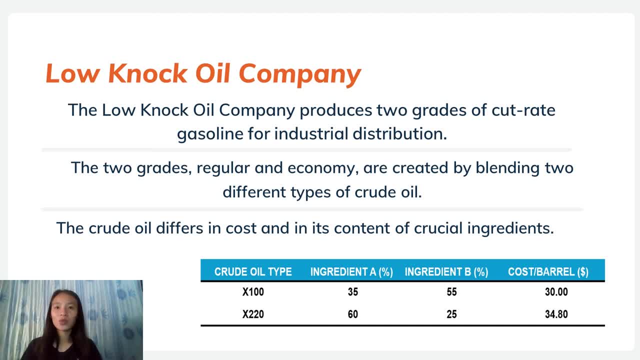 the objective is to minimize the cost. Each of the two types of gasoline has a demand constraint And each of the two types of gasoline has a constraint restricting the amount of the ingredients. Thus, there are four constraints. The decisions involve the amount of each type of crude oil. 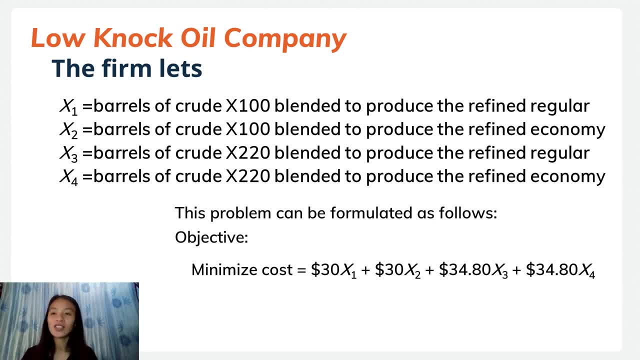 and the amount of each type of crude to use in each type of gasoline. So this will be the decision variables. let X1 be the barrels of crude X100 blended to produce the refined regular. X2 be the barrels of crude X100 blended to produce the refined economy. 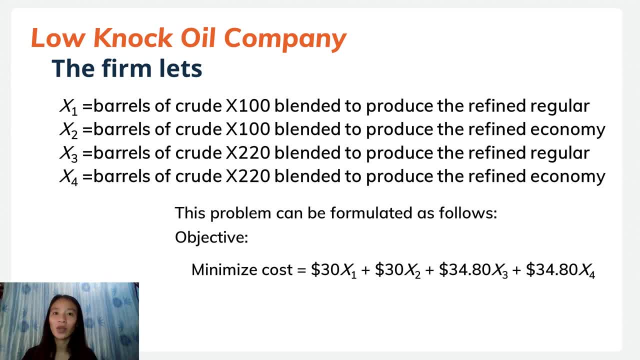 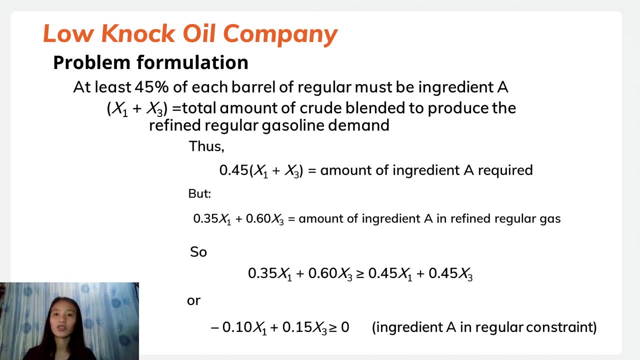 X3 be the barrels of crude X220 blended to produce the refined regular. X4 be the barrels of crude X220 blended to produce the refined economy. So this slide shows the computer the computation of ingredient A in the regular constraint And this slide shows the computation of ingredient B into economy constraint. 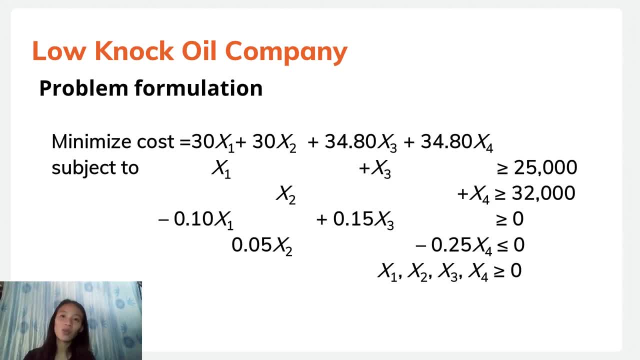 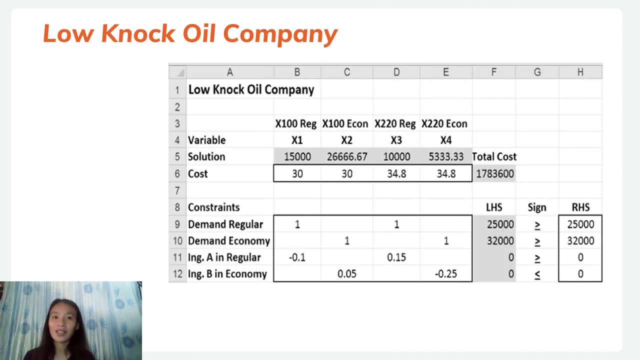 The objective of this problem is to minimize the cost. that is equals to the sum of $30 X1 plus $30 X2, plus $34.80 X3 plus $34.80 X4, and it is subject to the following constraints: Using the Excel. 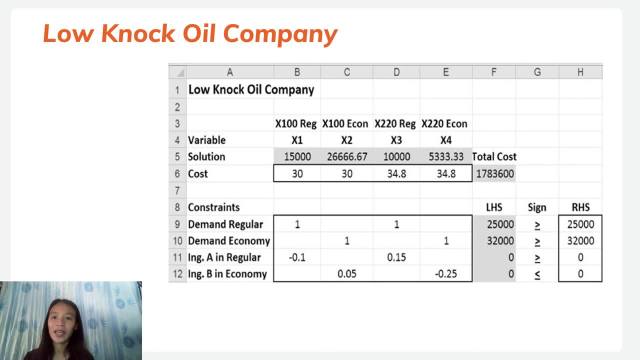 the solution to low NOC oil's formulation was found to be: X1 is equal to 15,000 barrels of X100 into regular. X2 is equals to 26,666.67 barrels of X100 into economy. X3 is equals to 10,000 barrels of X220 into regular. 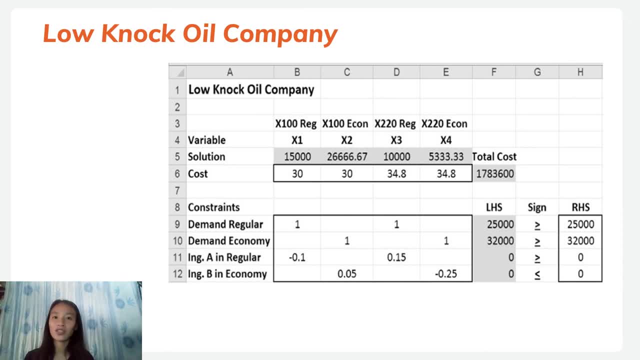 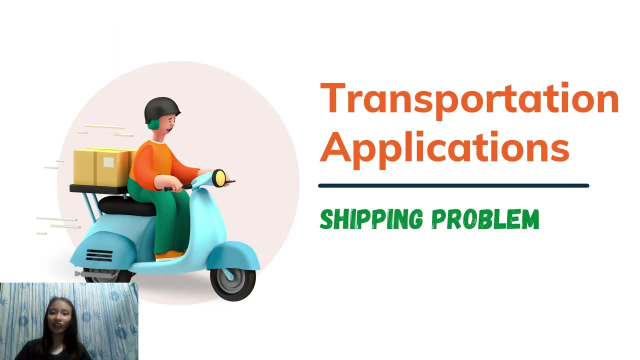 And X4 is equals to 5,333.33 barrels of X220 into economy And the cost of this mix is $1,783,600.. So the last topic for our report is about that: transportation applications, And under this application is the shipping problem. 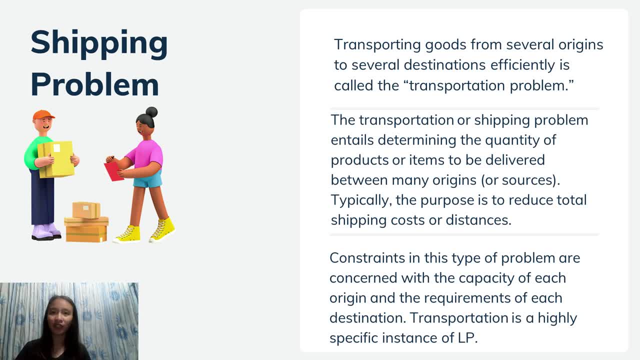 So transporting goods from several origins to several destinations efficiently is called the transportation problem, And the transportation or shipping problems entails determining the quantity of products or items to be delivered between many origins or sources. Typically, the purpose of this is to reduce total shipping cost or distances. 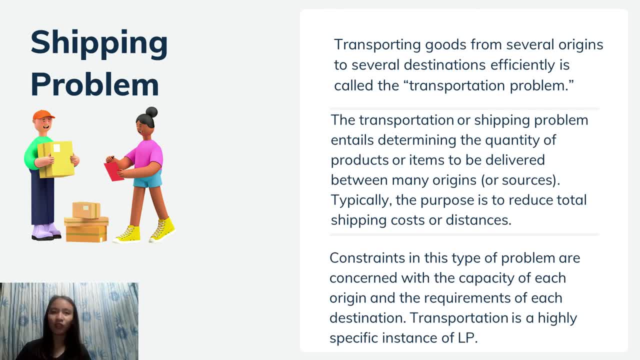 Constraints in this type of problem is concerned with the capacity of each origin and the requirement of each destination. Transportation is a highly specific instance of linear programming. Transportation problem is a special kind of linear programming problem in which the goods are transported from a set of sources to a set of destinations. 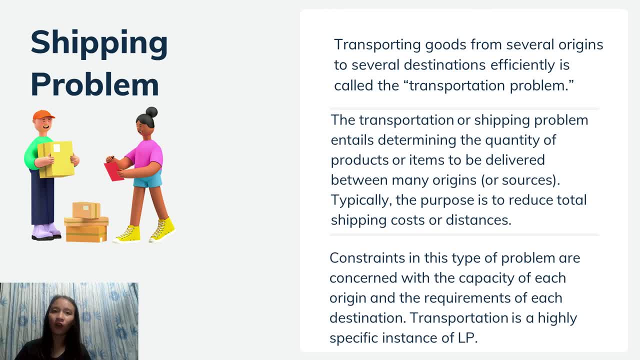 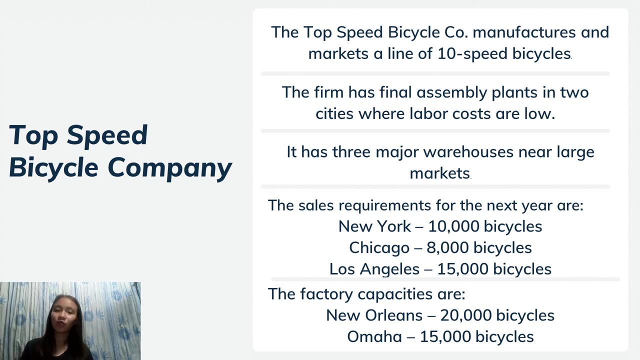 subject to the supply and demand of the sources and destinations respectively, such that the total cost of transportation is minimized. So let's use the Top Speed Bicycle Corporation as our example in this application. So the Top Speed Bicycle Corporation manufactures and markets a line of 10 speed bicycles. 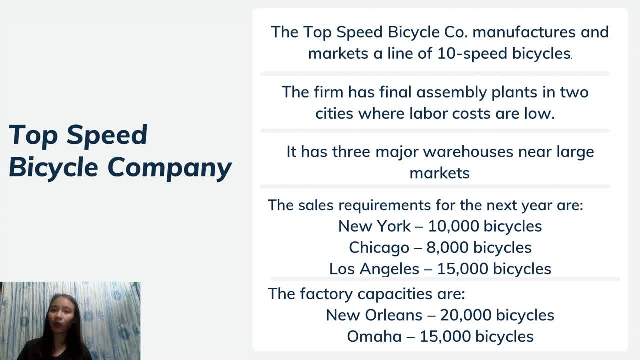 The firm has a final assembly plant in two cities where labor costs are low. It has three major warehouses near large markets. The sales requirements for the next year are 10,000 bicycles in New York, 8,000 bicycles in Chicago and 15,000 bicycles in Los Angeles. 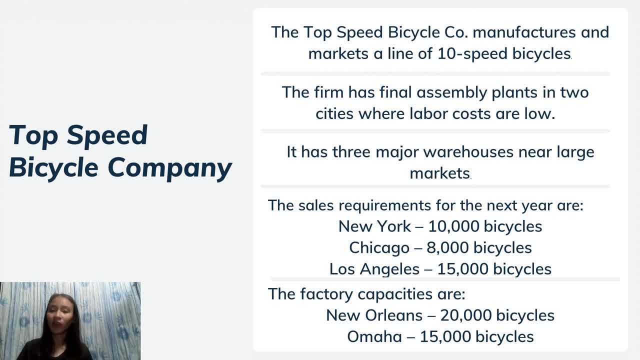 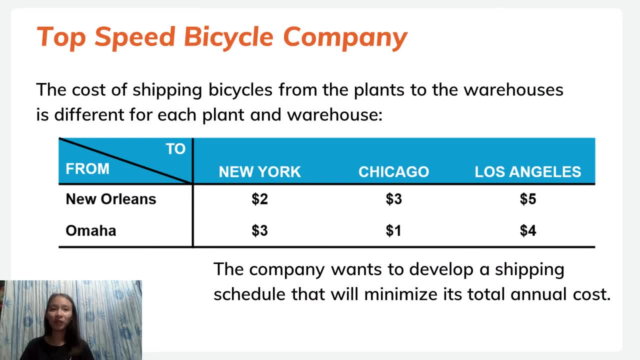 The factory capacities are 20,000 bicycles in New Orleans and 15,000 bicycles in Omaha. The cost of shipping bicycles from the plants to the warehouses is different for each plant and warehouses and it is shown in the table below. The company also wants to develop a shipping schedule that will minimize its total annual cost. 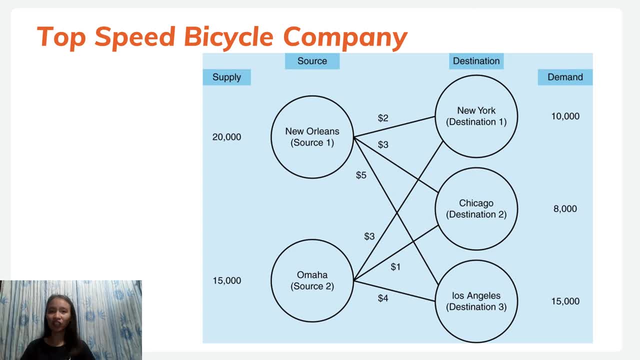 In this slide, the picture provides a network representation for this problem. Each circle represents source or a destination. in this problem, Each source and destination is numbered to facilitate a variable definition. Each arrow indicates a possible shipping route and the cost per unit to ship along each of these.